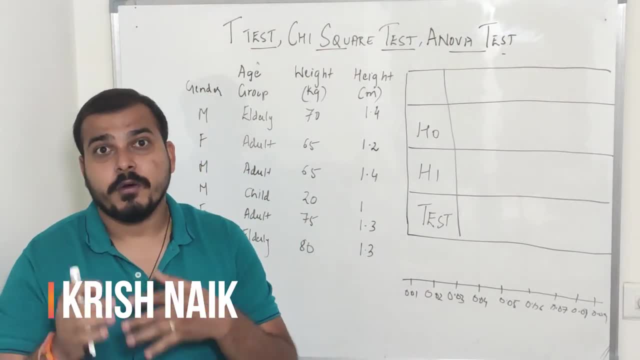 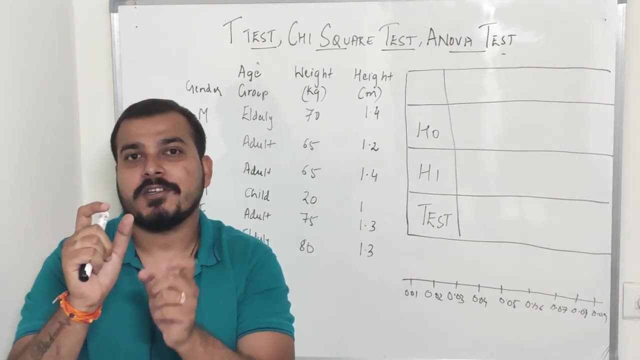 Hello all my name is Krishna and welcome to my YouTube channel. Today, in this particular video, we will be discussing about t-test, chi-square test, ANOVA test, and we will also be discussing about a very important thing which is called as p-value, which is also called as significance value. 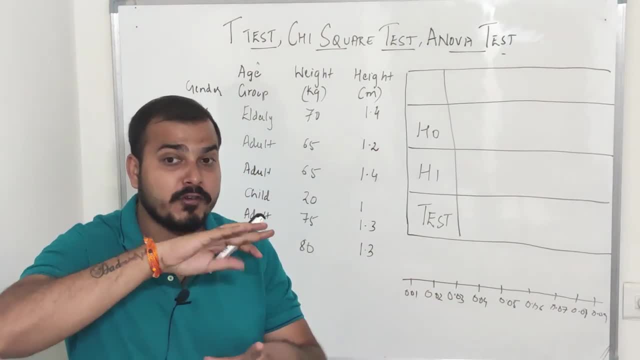 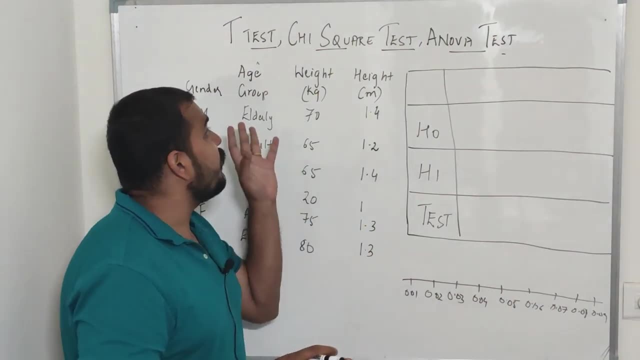 Now, guys, in my previous video, I have already explained you about hypothesis testing and I gave you your overall overview about it. We have discussed about null hypothesis, alternate hypothesis, But now, in this particular video, we will focus on when to use t-test, when to use chi-square test, when to use ANOVA test. 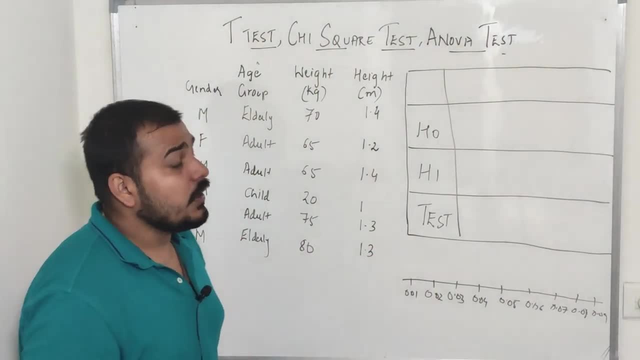 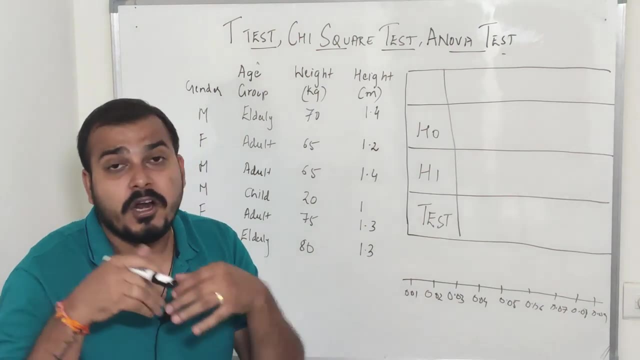 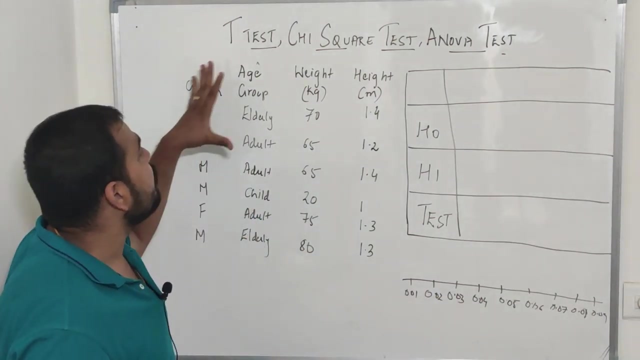 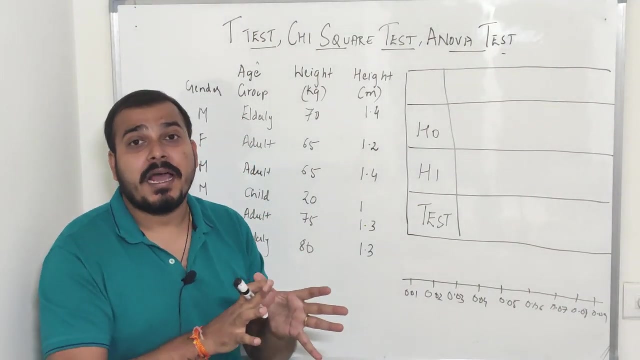 We are going to discuss about this. So, guys, and one more confusion that I usually get from students and some of my subscribers is that they are not able to relate this concept to the real world scenario. This is the main problem over here. So I am going to take a very simple data set over here and remember, guys, this is a sample of the data set and, as you remember, I told you that when we are discussing about hypothesis testing, we come to a conclusion for a population based on a sample data set. 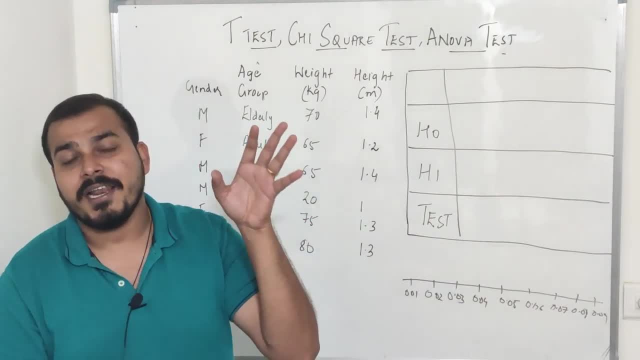 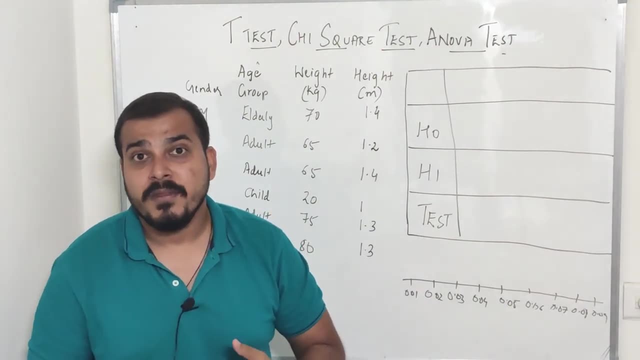 And, based on the sample data set, we will divide into alternate and null hypothesis and then we collect evidences and we apply different types of techniques and these are the other tests techniques that we can apply to find out whether null hypothesis is true or alternate hypothesis. 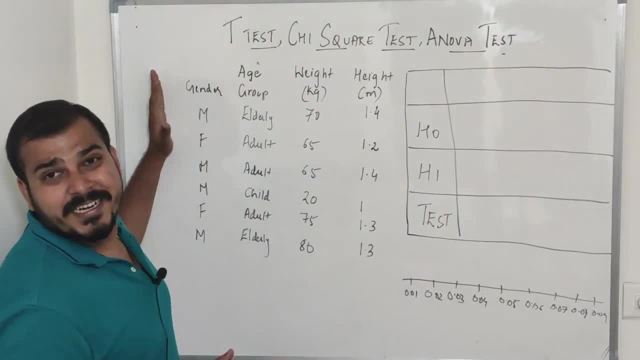 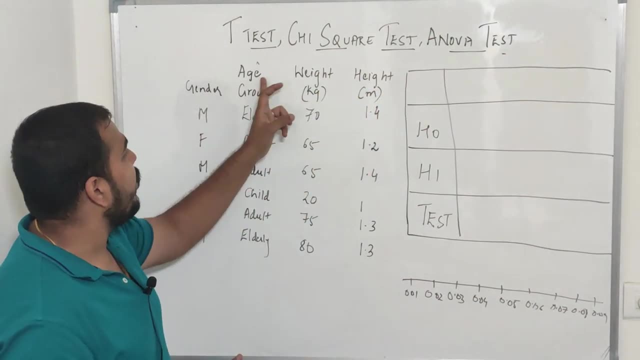 So let me go ahead and go a little over here. In this particular data set I have gender, age group, weight and height. Weight and height are gave as Kg and metres. Over here you have age group, which is my category feature. We have gender again. this is my category feature. Now let me consider and share this data set with you. I have e 2, i 2, that is, max 10, c 10 and 10.. You want to write this value below? All right. 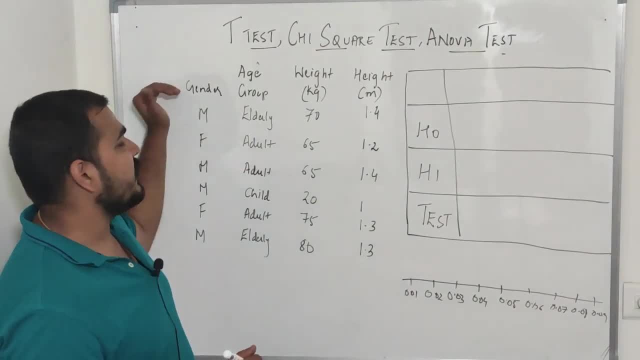 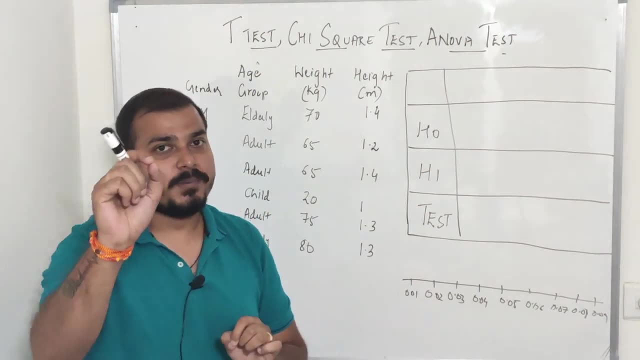 consider one category feature over here. So suppose I consider gender. Now what kind of conclusion, what kind of question, what kind of things I can research from this particular gender category. Just think in this particular example. I will just give you one simple example. 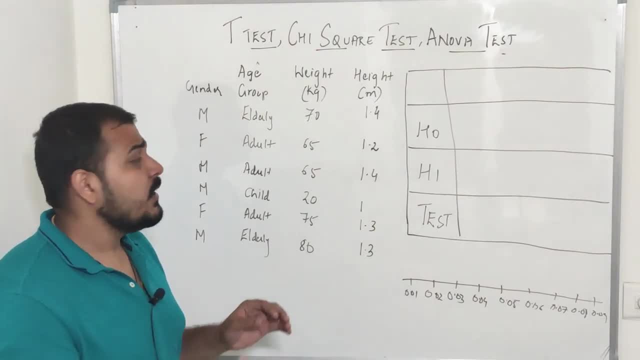 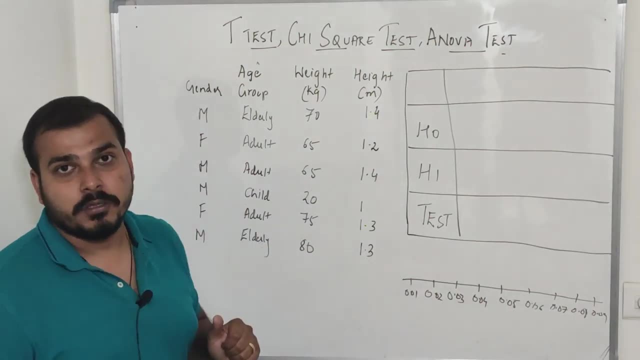 over here I will try to find out whether there is a difference in the proportion of male and female. So this is my question: Whether there is a difference between the proportion of male and female count. So what we do is that, in the hypothesis testing first of all, 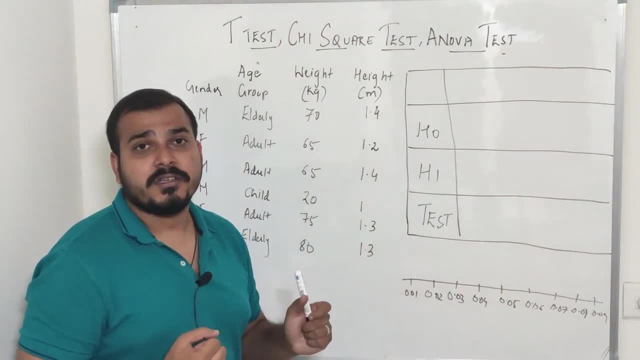 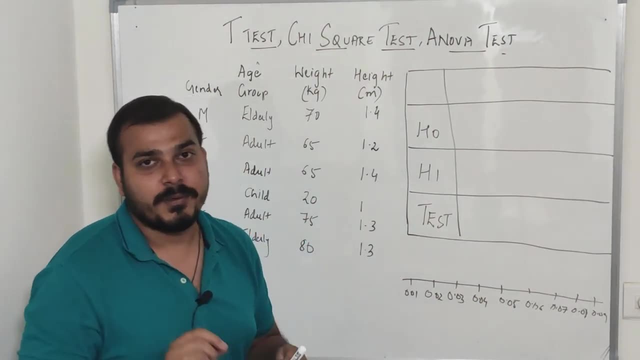 we need to consider our null hypothesis, then our alternate hypothesis, then we need to do a test on it and when this test, I will just be telling you what happens after this particular test. Now, in this particular case- alternate hypothesis- I will just say that 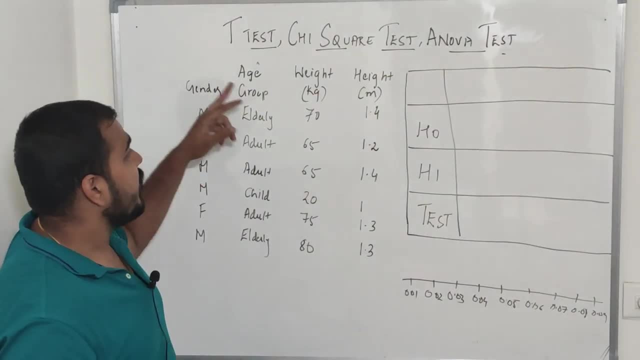 So let us go ahead. So in this particular data set I have genders, age group, weight, height. Weight and height are given in kg and meters over. here you have age group, which is my category feature. we have gender, again, this is a category feature. 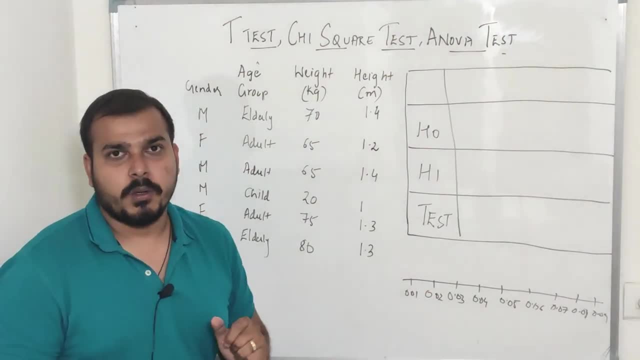 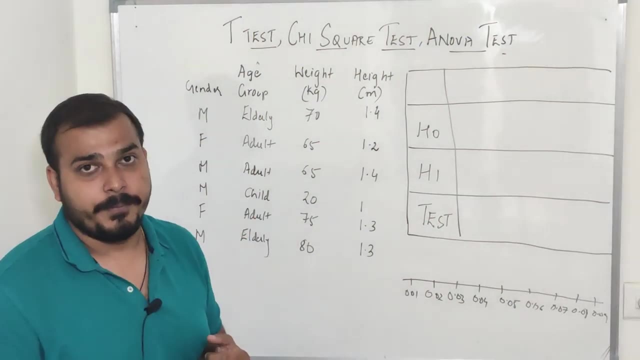 Now let me just consider a system, one category feature over here. So suppose I consider gender. Now what kind of conclusion, what kind of question, what kind of things I can research from this particular gender category. Just think in this particular example. I will just give you one simple example over. 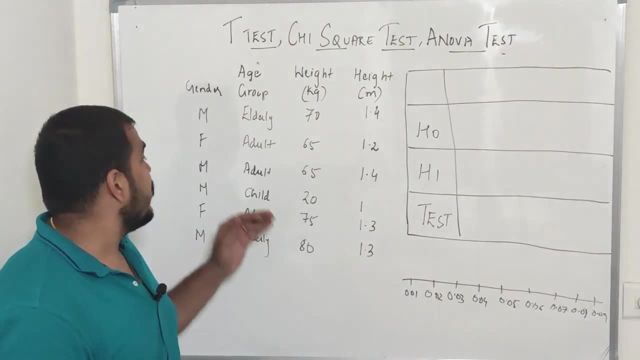 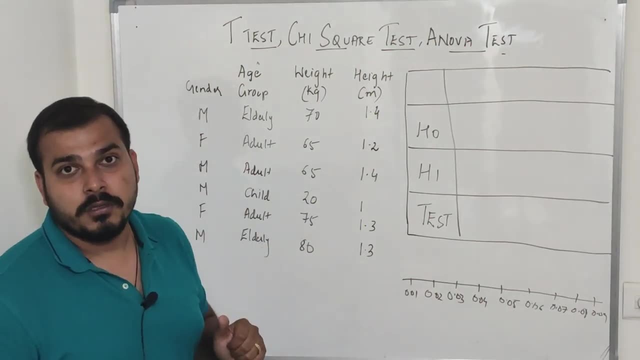 here I will try to find out whether there is a difference in the proportion of male and female. So this is my question: Whether there is a difference between the proportion of male and female count. So what we do is that, in the hypothesis testing first of all, 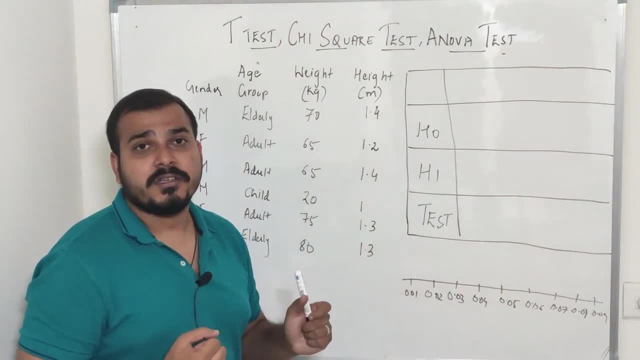 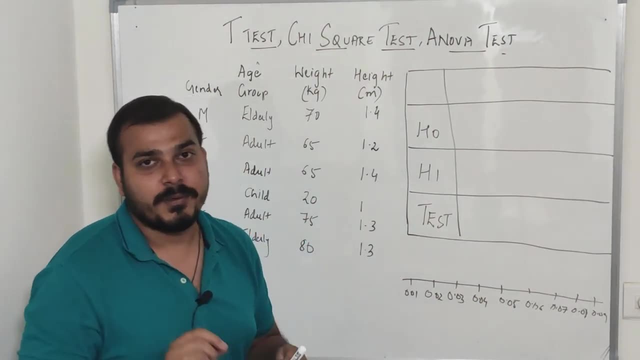 we need to consider our null hypothesis, then our alternate hypothesis, then we need to do a test on it and when this test, I will just be telling you what happens after this particular test. Now, in this particular case- alternate hypothesis- I will just say that 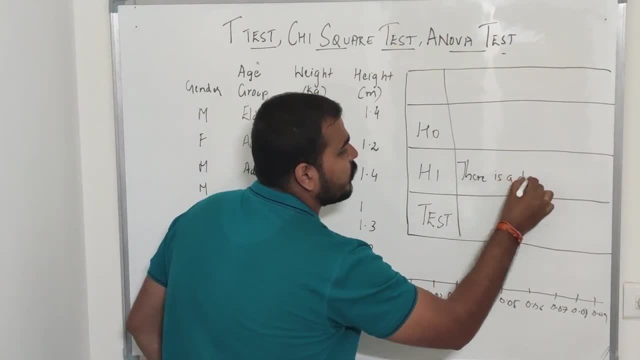 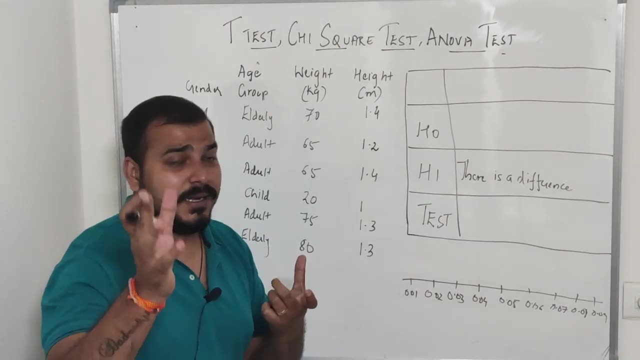 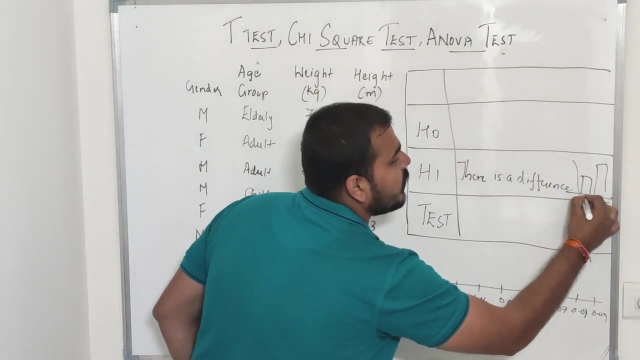 yes, there is a difference. There is a difference in the proportion. Suppose this is my alternate hypothesis. Now, always remember, guys, there is a difference. Now suppose if I just take this sample data set, if I just create a plot diagram, A barge plot like this for male and female, Then, considering this barge chart, I can come. 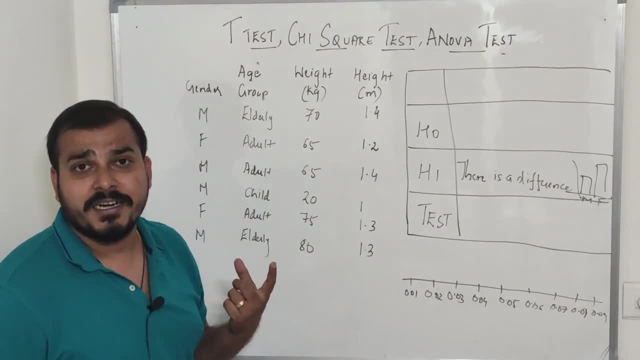 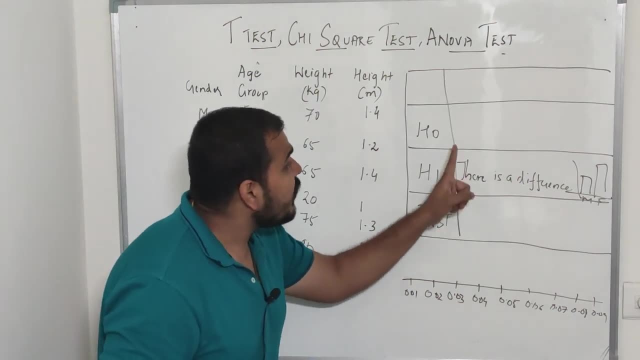 to know that, whether there is a difference in the proportion of male and female from this particular data set. But remember guys, this is just a sample data set. It is not a population data set, So for that reason we also have to consider a null hypothesis. 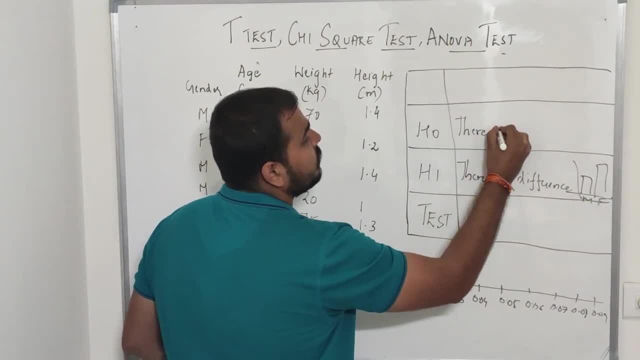 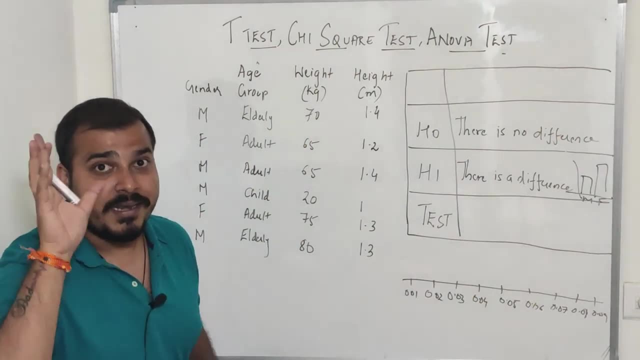 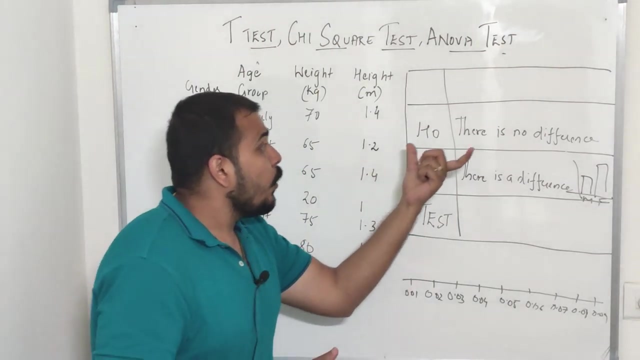 So null hypothesis will be that there is no difference. So this is my null hypothesis, which will always be true. Now, considering any test over here, considering one particular feature, I will need to apply a test which says that, where we have this null hypothesis as true, what is the likelihood? 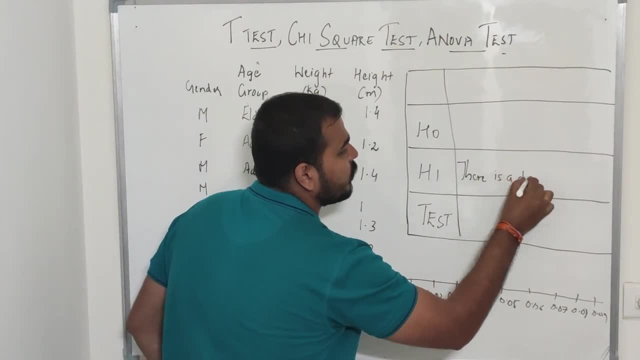 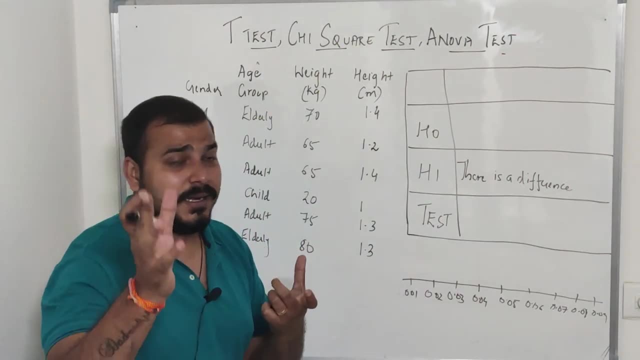 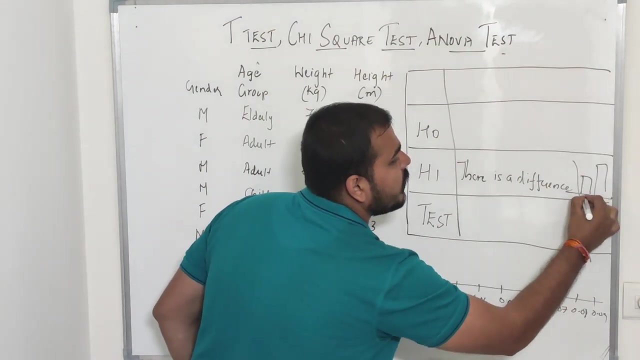 yes, there is a difference. There is a difference in the proportion. Suppose this is my alternate hypothesis. Now, always remember, guys, there is a difference. Now suppose if I just take this sample data set, if I just create a plot diagram, A barge plot like this for male and female, Then, considering this barge chart, I can come. 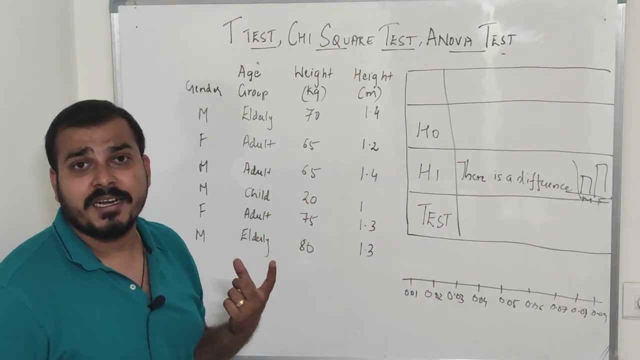 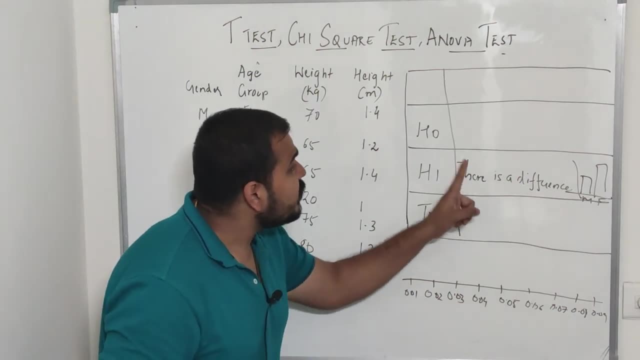 to know that, whether there is a difference in the proportion of male and female from this particular data set. But remember guys, this is just a sample data set. It is not a population data set, So for that reason we also have to consider a null hypothesis. 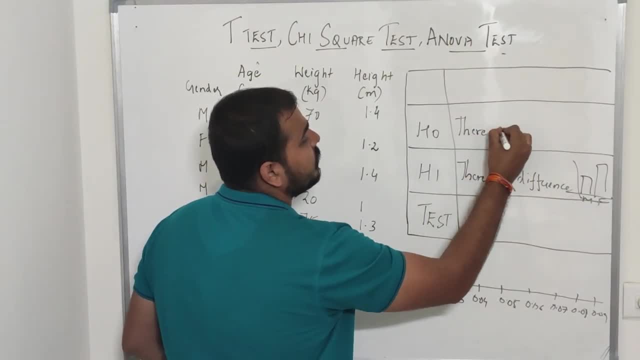 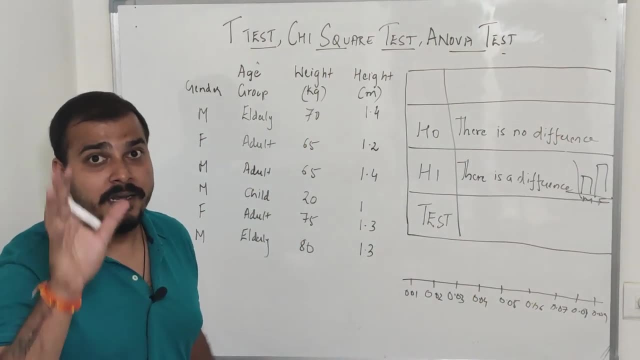 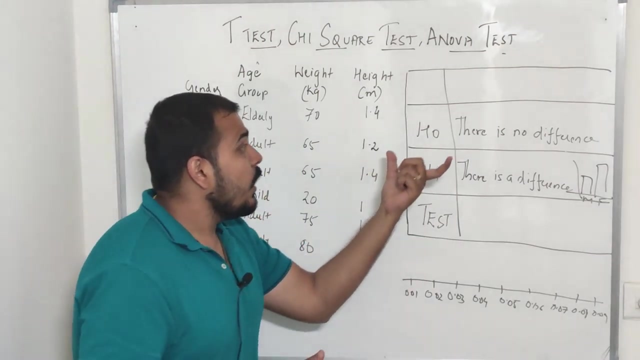 So null hypothesis will be that there is no difference. So this is my null hypothesis, which will always be true. Now, considering any test over here, considering one particular feature, I will need to apply a test which says that, where we have this null hypothesis as true, what is the likelihood? 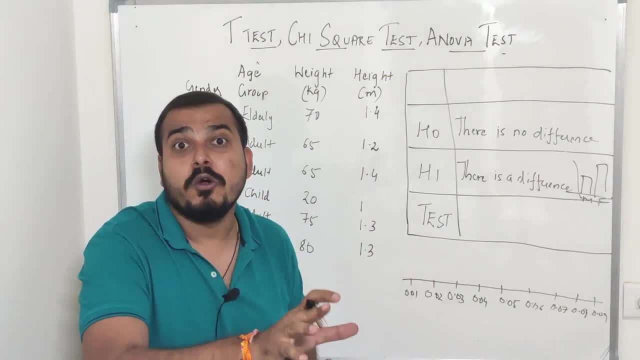 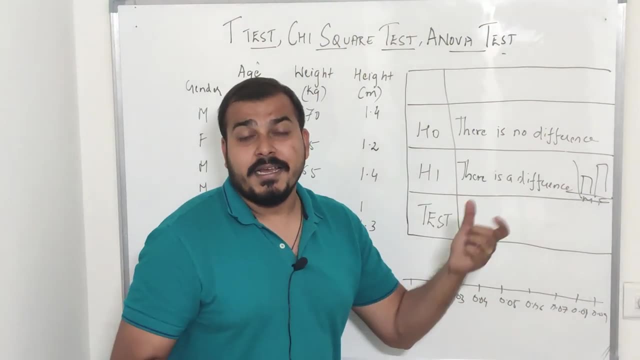 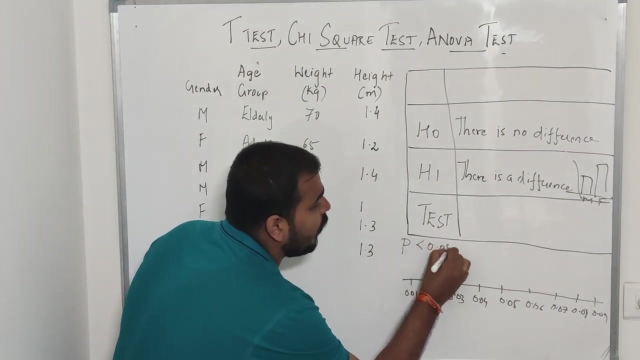 that your alternate hypothesis will be true. What is your likelihood or what is your probability that your alternate hypothesis will be true, Considering your null hypothesis is true, And when I do this particular test and for this particular test, suppose I get, the value p is less than 0.05.. 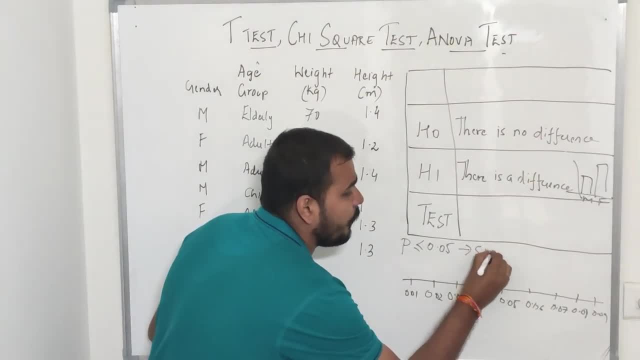 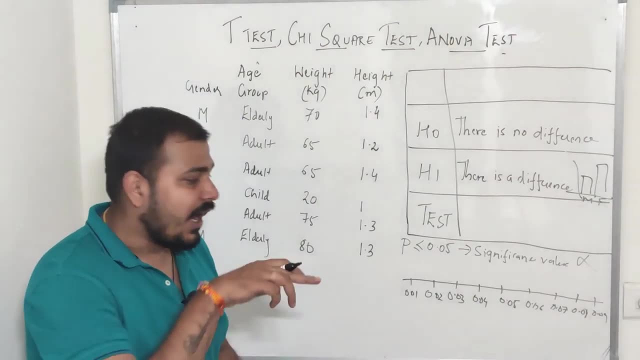 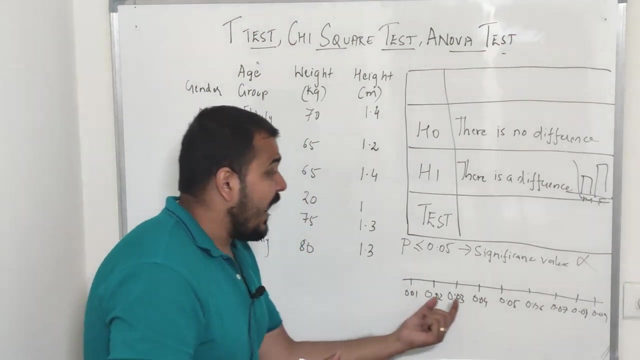 Now, in this particular p value is basically called as significance value, Significance value. it is also mentioned as alpha, So we consider a significance value like 0.05.. Again, I will explain you. what is the significance value, what does it say? And after applying, 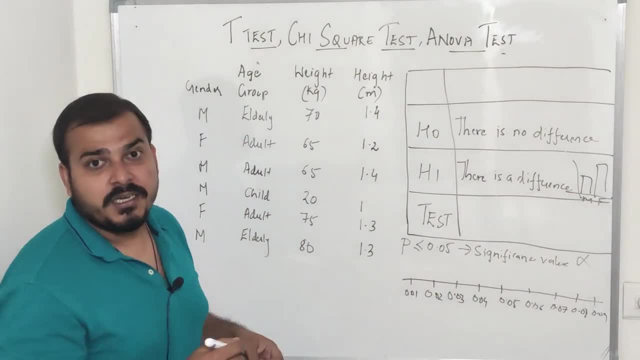 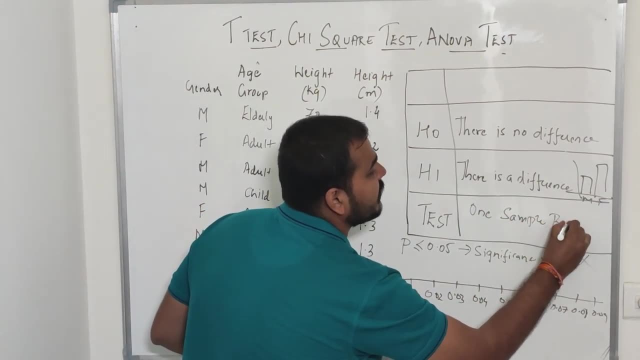 this particular test. now, since we have just taken one category feature, the type of test that we basically apply is something called as one sample proportion test. One sample proportion test. Okay, guys, just understand this, because in my upcoming classes I will be telling you: 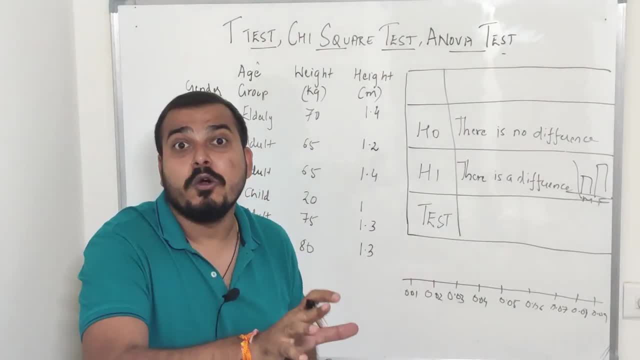 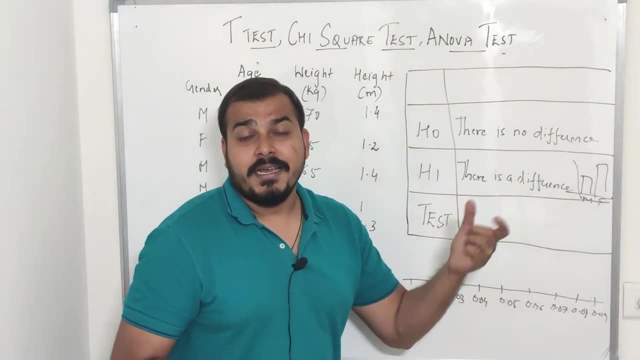 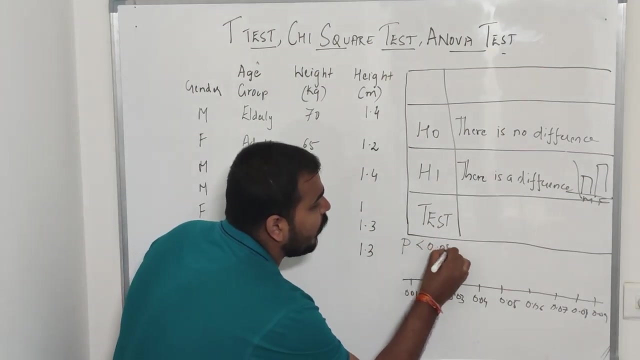 that your alternate hypothesis will be true. What is your likelihood or what is your probability that your alternate hypothesis will be true, Considering your null hypothesis is true, And when I do this particular test and for this particular test, suppose I get, the value p is less than 0.05.. 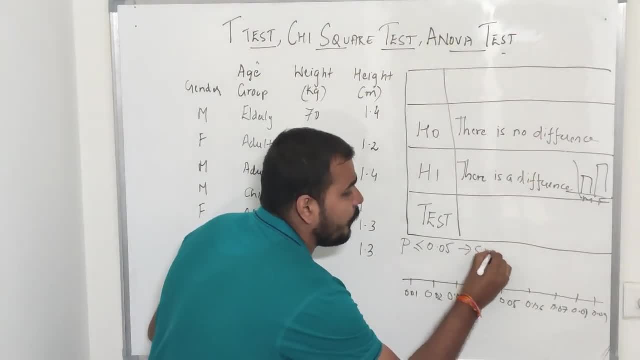 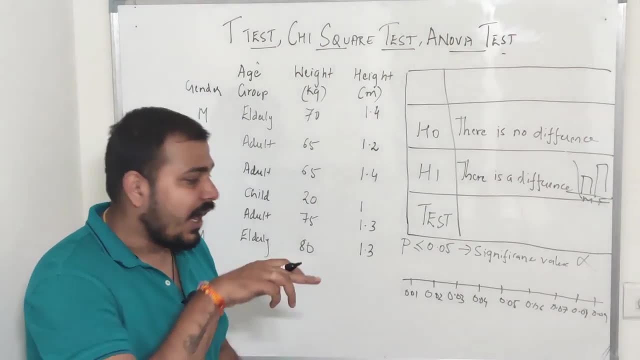 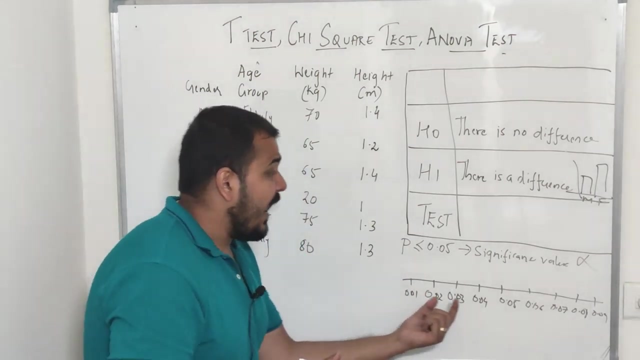 Now, in this particular p value is basically called as significance value, Significance value. it is also mentioned as alpha, So we consider a significance value like 0.05.. Again, I will explain you. what is the significance value, what does it say? And after applying, 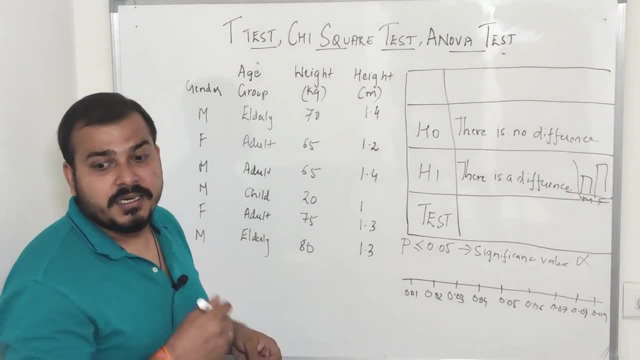 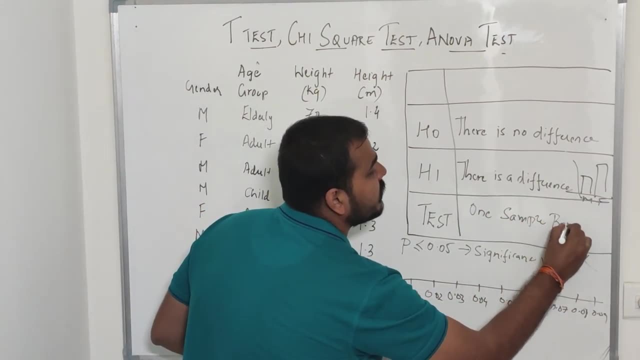 this particular test. now, since we have just taken one category feature, the type of test that we basically apply is something called as one sample proportion test. One sample proportion test. Okay, guys, just understand this, because in my upcoming classes I will be telling you: 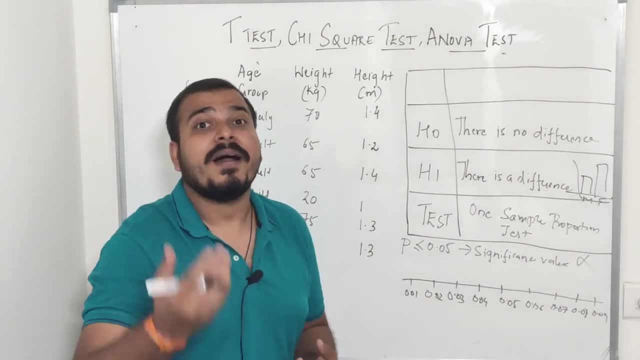 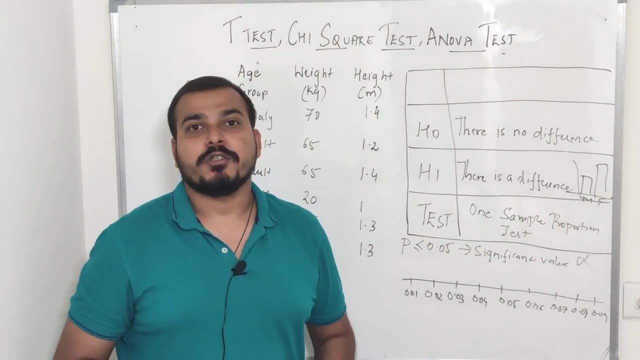 the mathematical formula for this, how you can do with the help of python also. But just consider that if you are just considering one category feature, the type of test that you have to use is called as one sample proportion test, And let me write over here as one category. 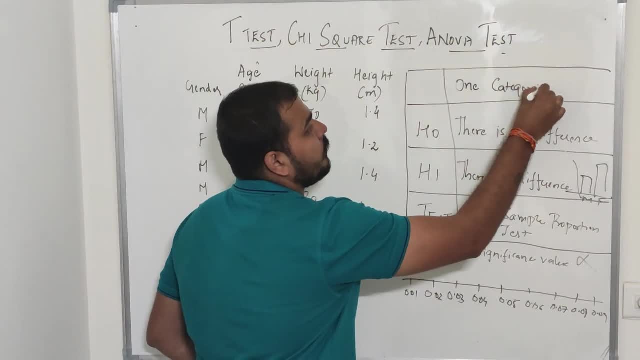 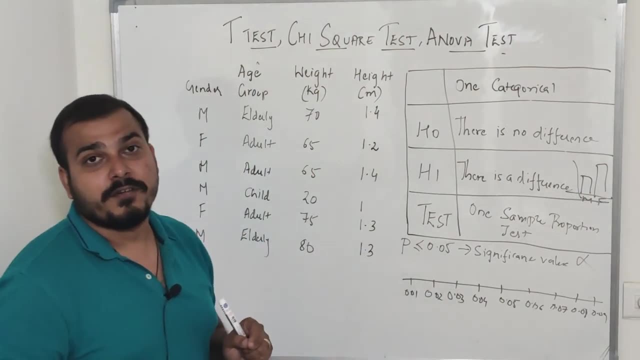 feature, One category. Okay, So suppose if I have one category feature, then I basically need to apply one sample proportion test and if I get my p value less than 0.05.. Now, always remember guys, this p value needs to be equal to 0.05.. So if I get my p value less than, 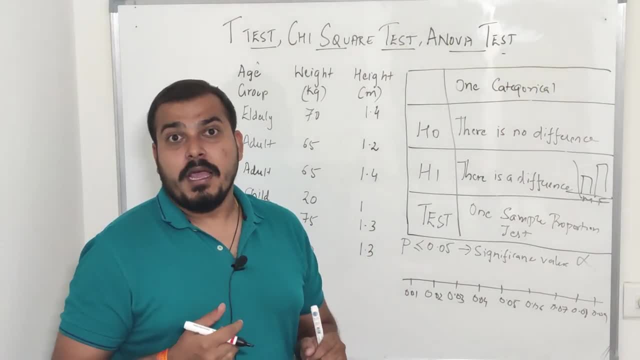 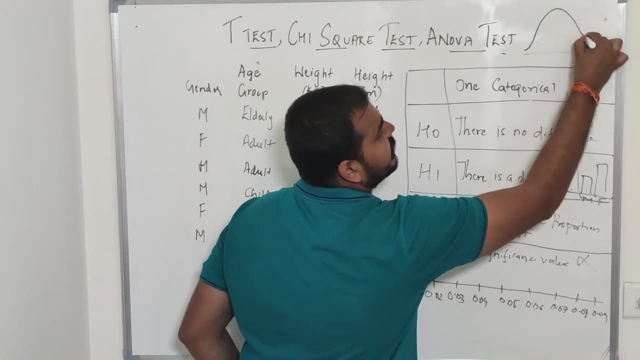 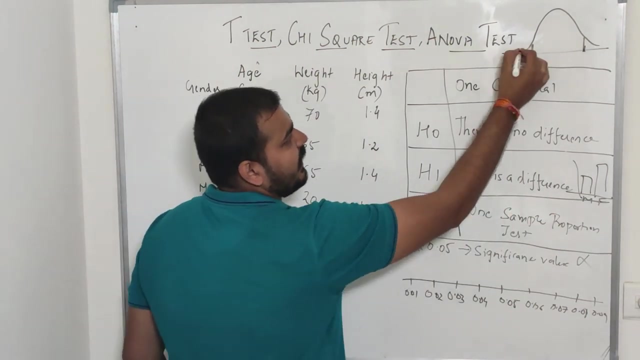 0.05, the function is selected before this particular test is basically done. Okay, Why 0.05?? Just understand in this particular way: If we take 0.05, suppose we have Gaussian distribution somewhere like this- Okay, Then we are basically considering that if our test says that it falls in this tail, 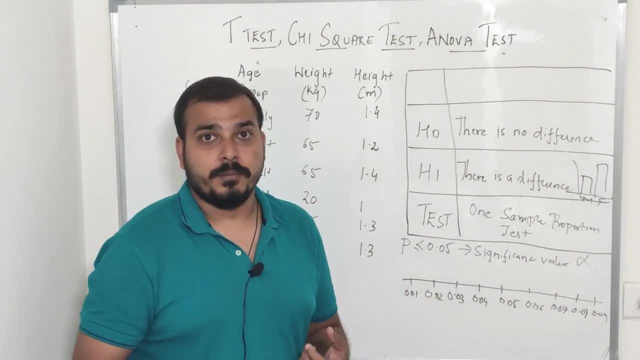 the mathematical formula for this, how you can do with the help of python also. But just consider that if you are just considering one category feature, the type of test that you have to use is called as one sample proportion test, And let me write over here as one category. 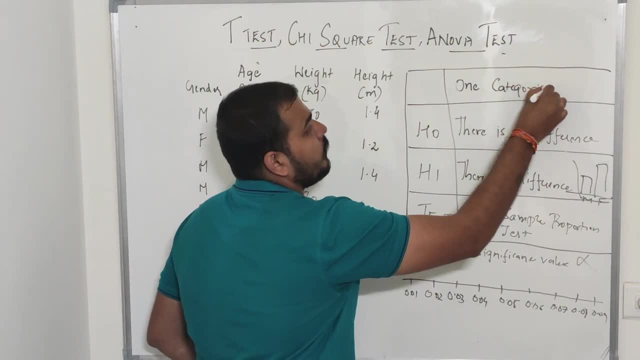 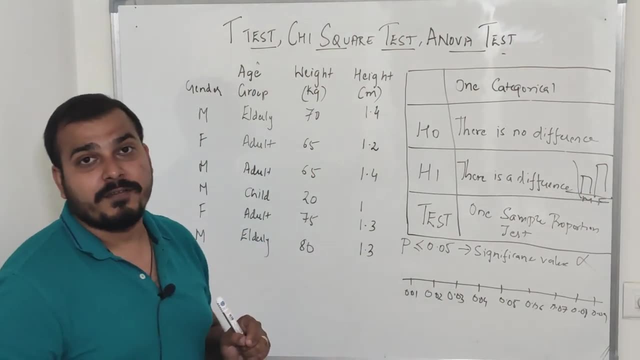 feature One category. Okay, So suppose if I have one category here, then I basically need to apply one sample proportion test and if I get my p value less than 0.05.. Now, always remember guys, this p value needs to be equal to 0.05.. So if I get my p value less than, 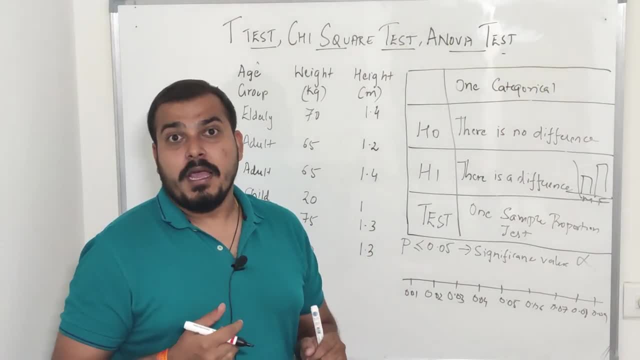 0.05, then I cannot apply one way is because water lower than 0.05 for one category features that you are not going to be able to do right рав. So that isрам fabric aén. stable material room sayov. So this will become the form that. 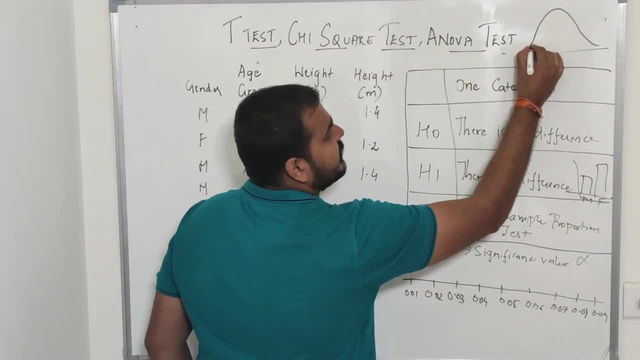 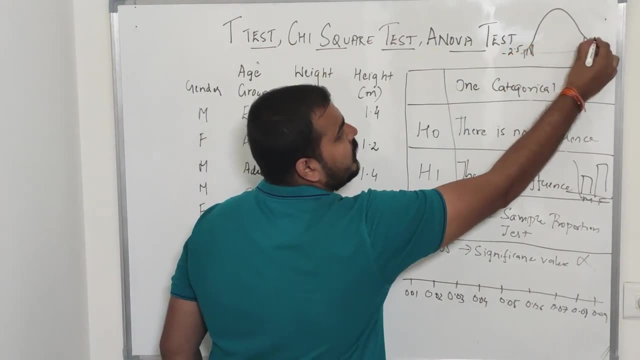 we used for formula of by dlategoi. So y'all, reasonably speaking, for the purpose of my graphics, for all of my police drawing d area which was selected before this particular test is basically done. Okay, why 0.05,? just? 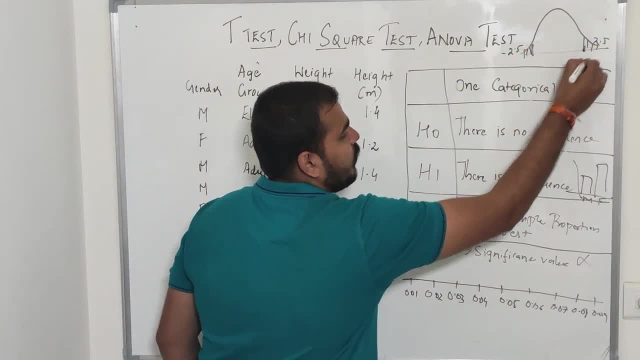 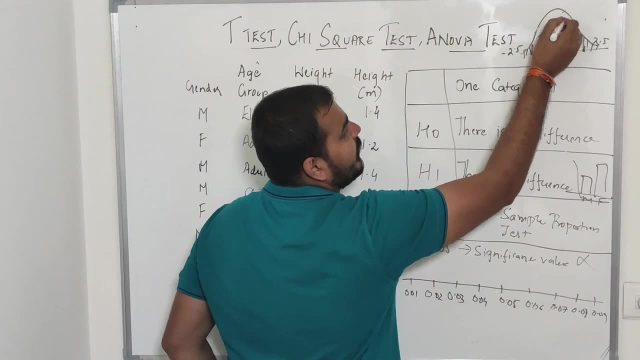 region like 2.5 over here. 2.5 over here, Okay. 0.05 basically means 5% of the total distribution. test to fall somewhere here. if it is less than 0.05, we are considering that it is. 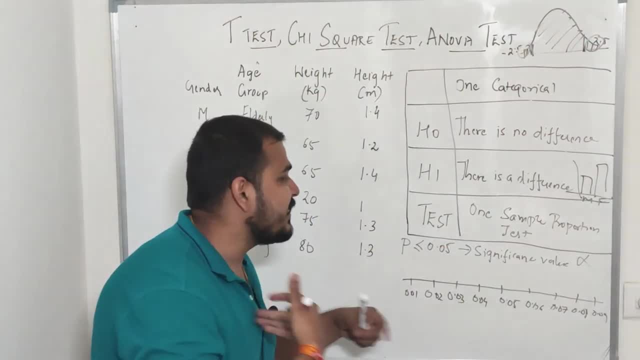 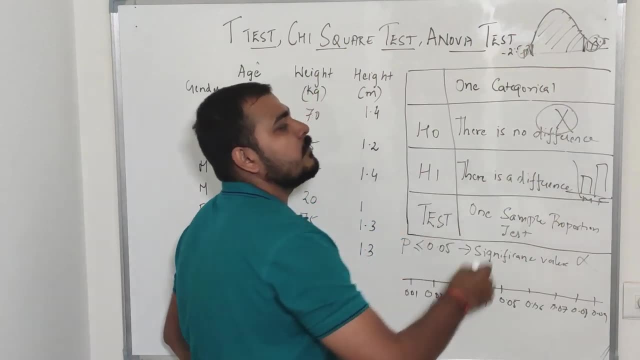 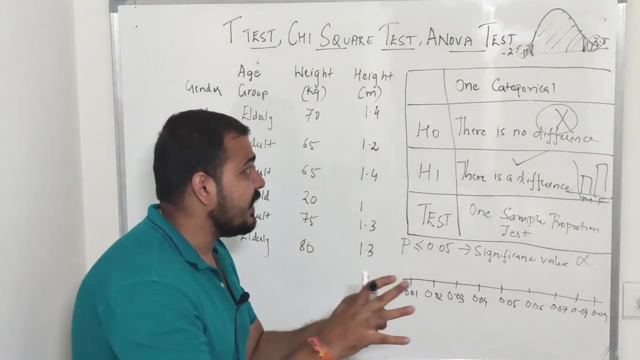 falling in this tail region. okay, so we are actually rejecting it. okay, now, if your p-value is less than 0.05, we are going to reject the null hypothesis and then we are going to accept the alternate hypothesis. okay, this basically comes in now. see, understand, guys? we have considered that the null hypothesis is. 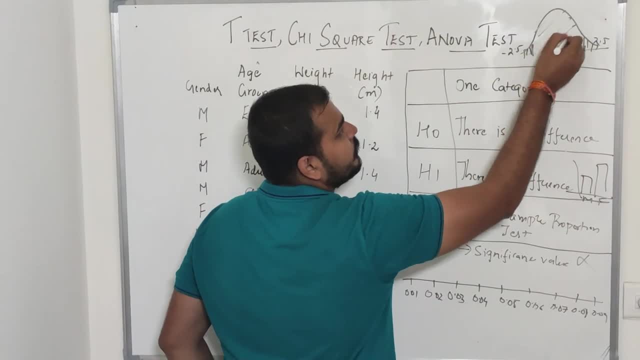 understand in this particular way. If you take 0.05- suppose we have Gaussian distribution somewhere like this, okay, Andwe are basically considering that if our test says that it falls somewhere here, if it is less than 0.05, we are considering that it is falling in this tail region. 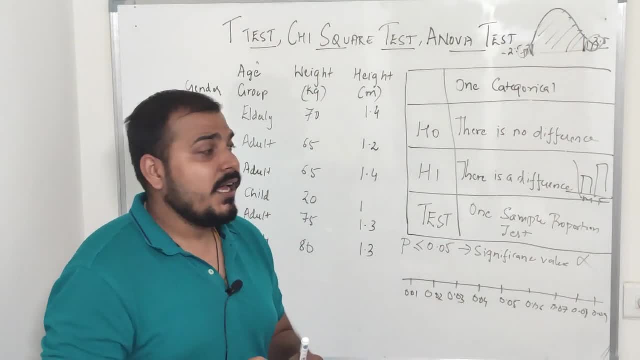 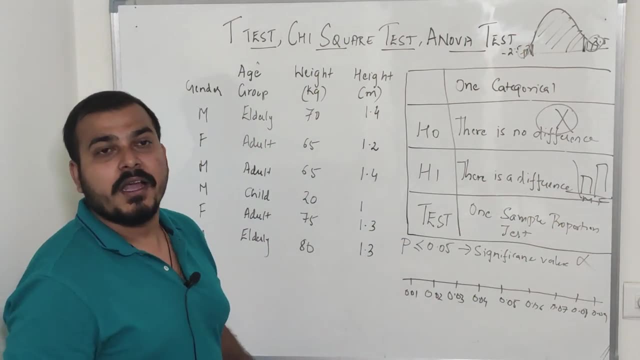 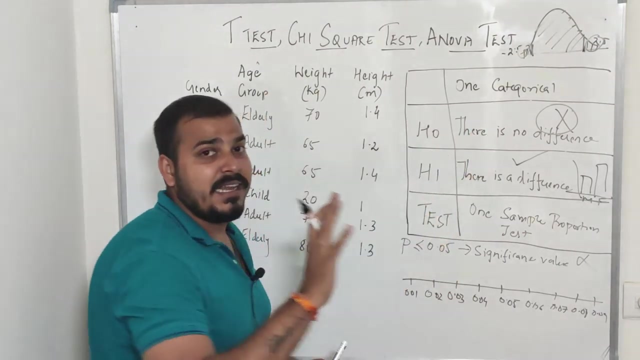 okay, so we are actually rejecting it. okay, now, if your p value is less than 0.05, we are going to reject the null hypothesis, and then we are going to accept the alternate hypothesis. okay, this basically comes in now. see, understand, guys, we have considered that the null hypothesis is true. 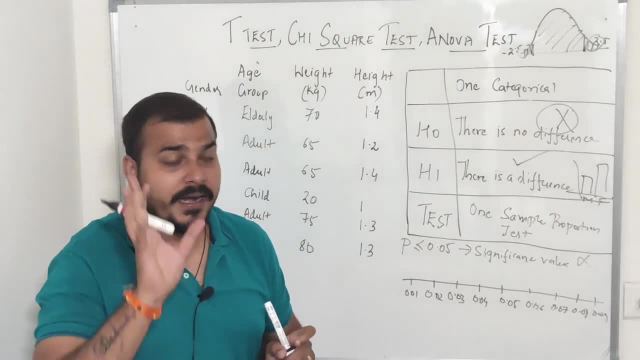 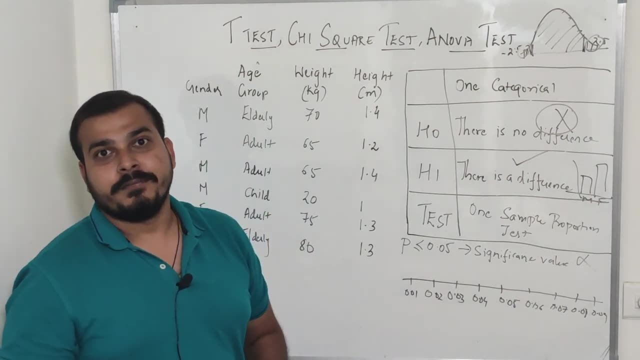 now, what is the likelihood that my alternate hypothesis will be true, right and based on that, the type of test you do, if you are considering one category feature is something called as one sample proportion test. and if this particular test gives me a value less than 0.05, okay, somewhere. 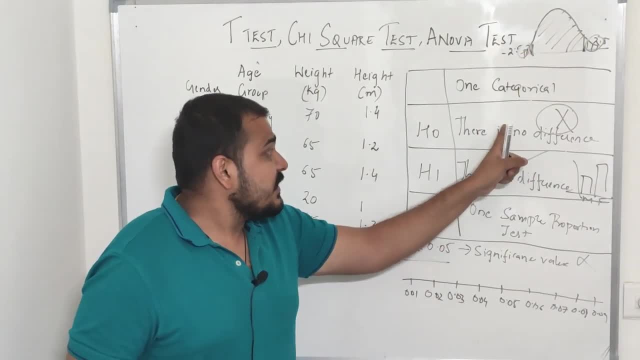 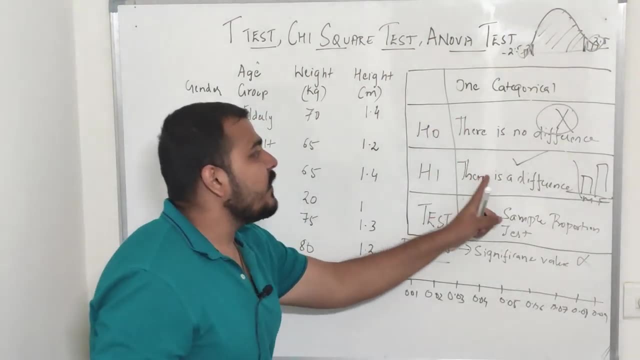 here that i am going to reject this because this is not supporting it. we have a very small value, somewhere less than 0.05, right? so we need to reject the null hypothesis and then we need to accept the alternate hypothesis, and then we will consider that there is a difference between the 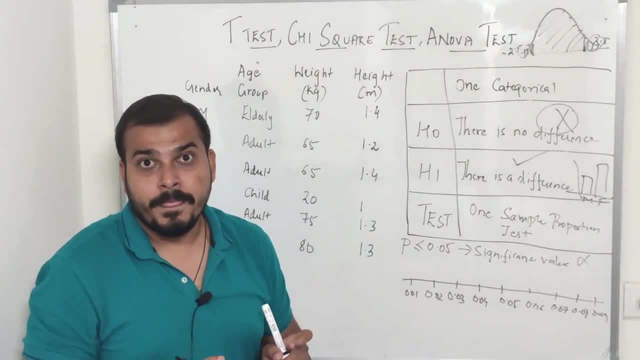 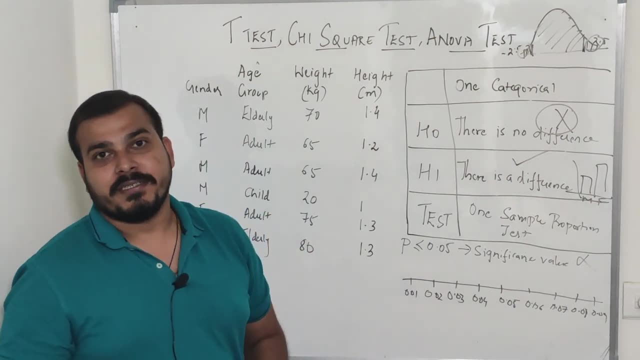 true. now what is the likelihood that my alternate hypothesis will be true? right, and based on that, the type of test you do, if you are considering one category feature is something called as one sample proportion test, and if this particular test gives me a value less than 0.05, okay, somewhere here that I am. 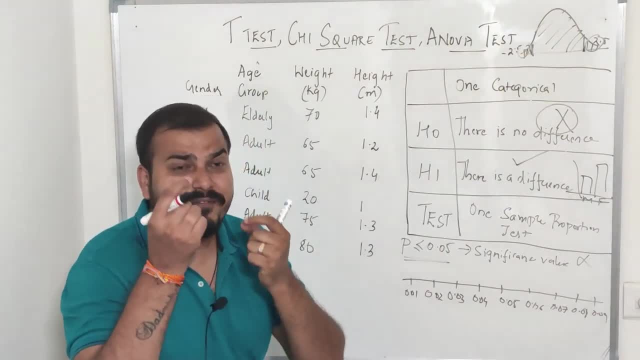 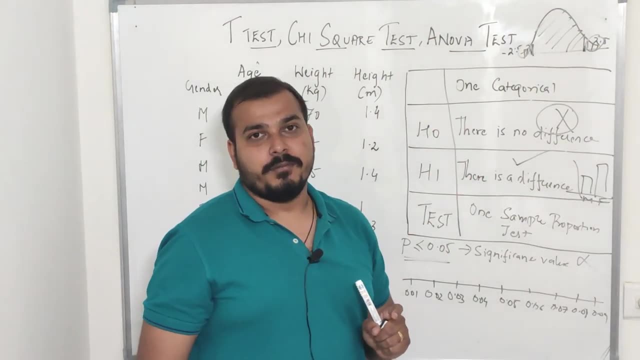 going to reject this, because this is not supporting it. we have a very small value, somewhere less than 0.05, right? so we need to reject the null hypothesis and then we need to accept the alternate hypothesis, and then we will consider that there is a difference between the proportion of the count in the male and female. 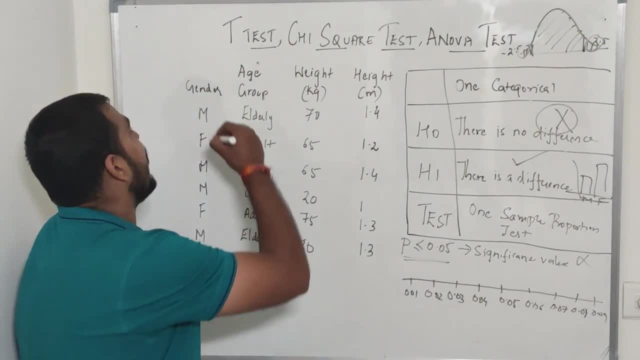 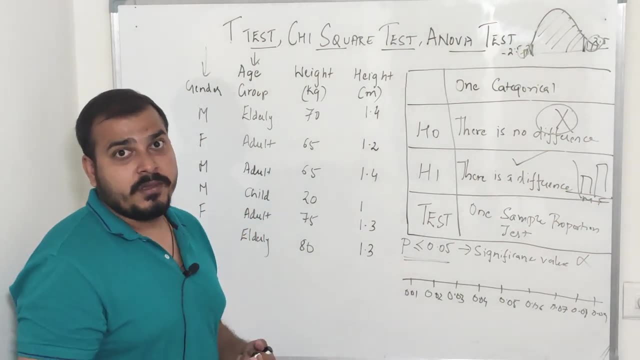 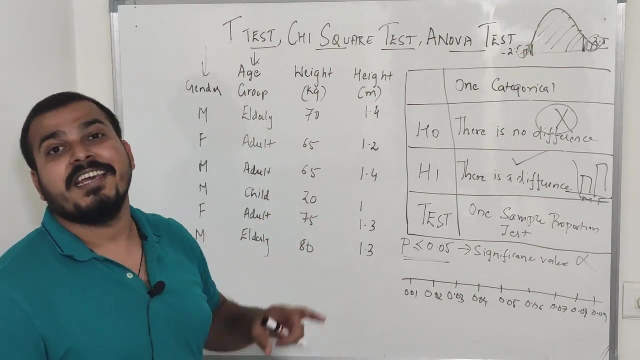 test ratio. okay, now, suppose if I take two category feature, suppose I take two category feature now. okay, now what kind of question may come with respect to two category feature? so with respect to two category feature, I may say, that is, there is a difference between male and female proportion based on age group. okay, based. 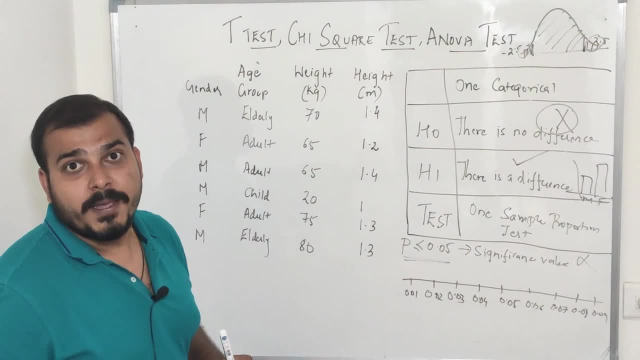 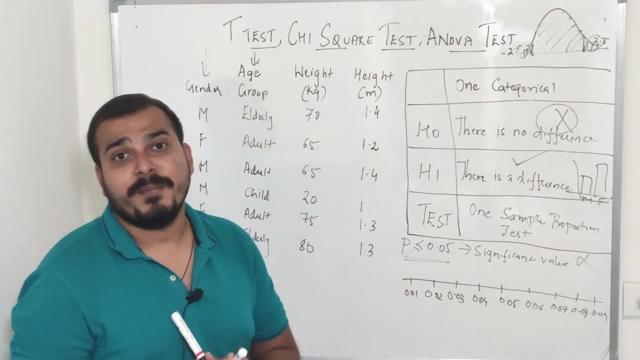 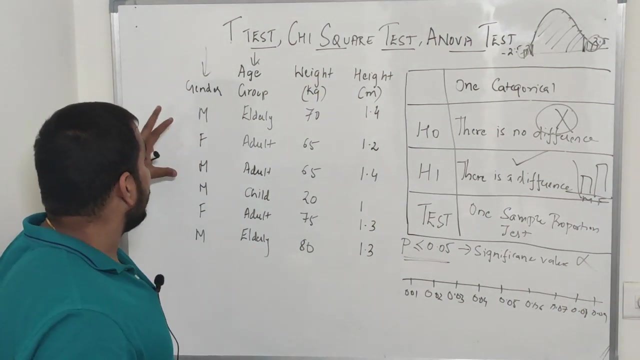 proportion of the count in the male and female ratio. okay, now suppose if i take two category feature. suppose i take two category feature now. okay, now what kind of question may come with respect to two category feature? so with respect to two category feature i may say that is, there is a difference between male and female proportion based on age. 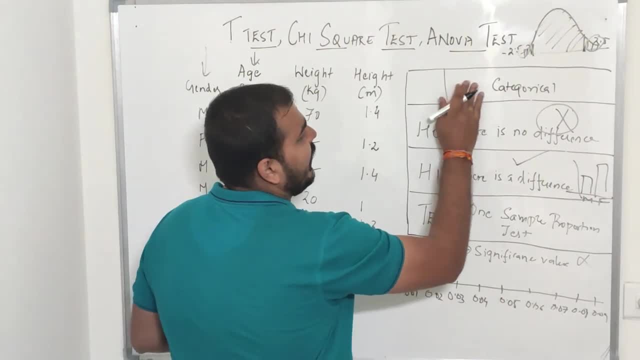 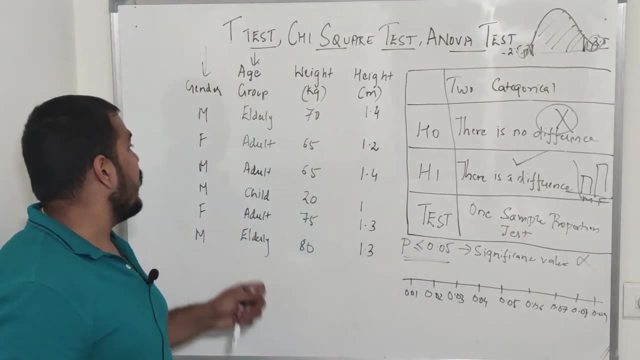 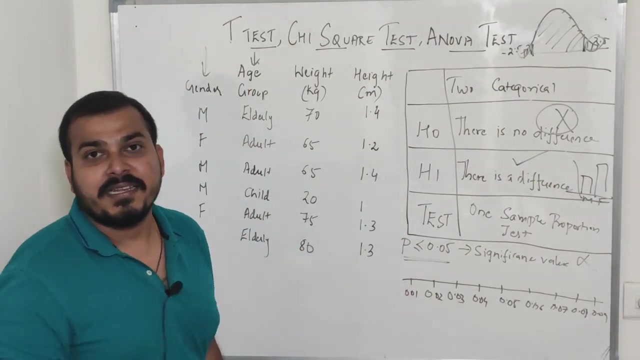 group. okay, based on age group. now this one category become two category, right. okay, now again i can again construct this particular bar plot based on this age group and all again. my hypothesis will be that there is a difference and my null hypothesis says that there is no. then 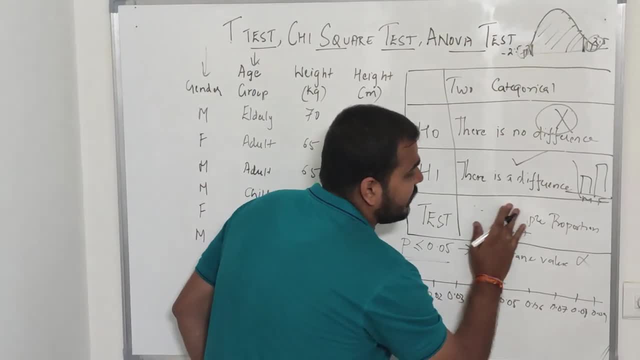 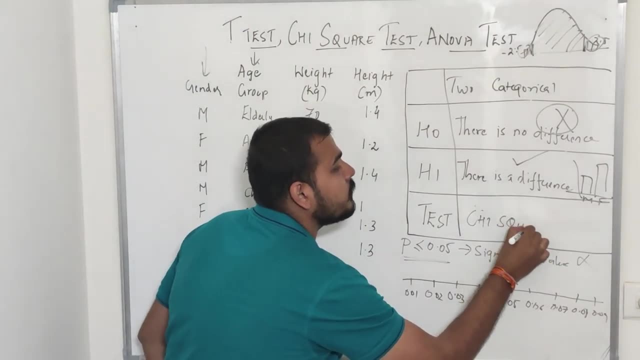 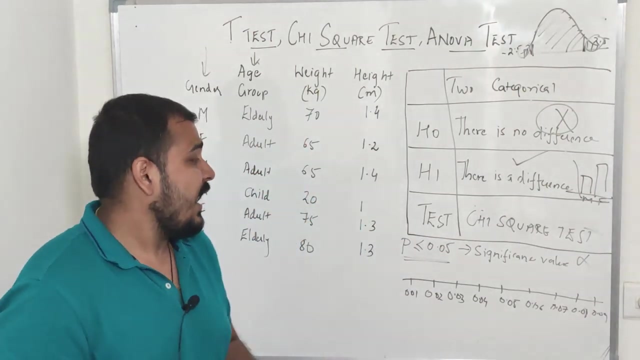 there will be no difference. right then, the type of test that we apply if we have two category feature is something called as chi square test. now, if this chi square test gives us a value less than 0.05, at that time we are going to consider. 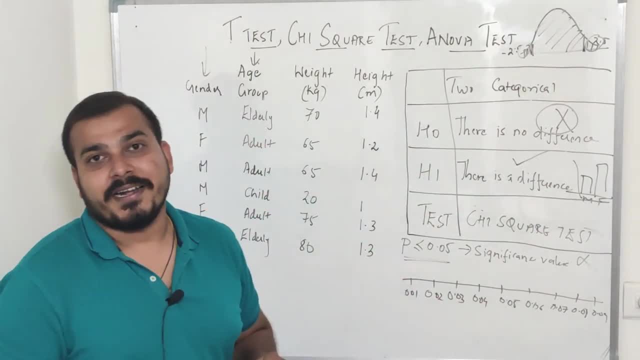 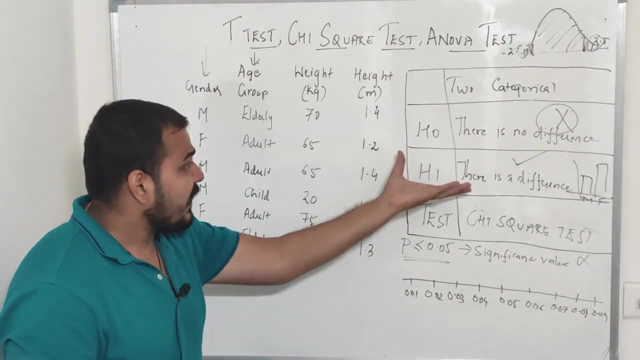 it that we are going to reject the null hypothesis and accept the alternate hypothesis? always remember, guys, if you are using two category feature and if you are trying to come to a conclusion, like a statement that i've actually told right at that time, you basically have to use a chi square test. 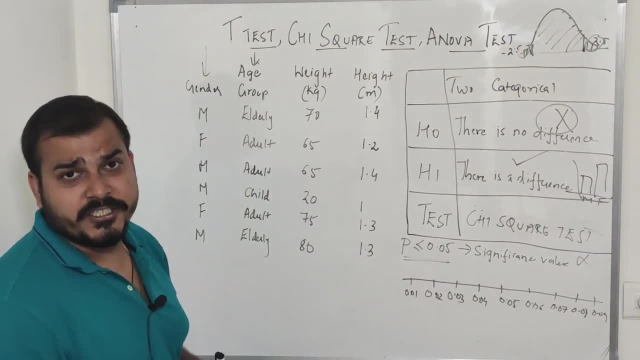 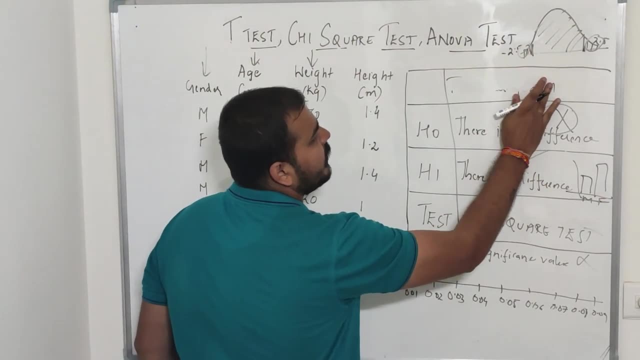 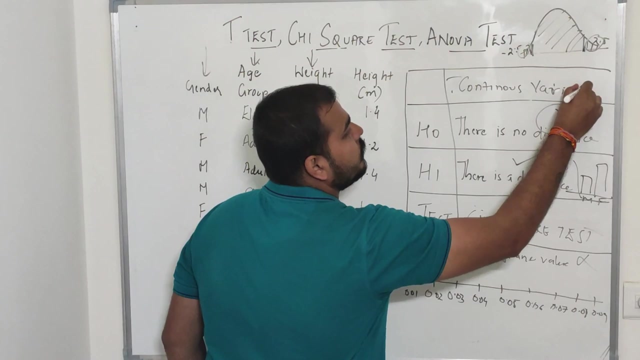 okay, now. now, instead of category feature, let me consider one continuous numerical value. okay, now, this two category. i'll just remove it, and let me just say that. one continuous variable. What kind of statement can come up with respect to this continuous variable? 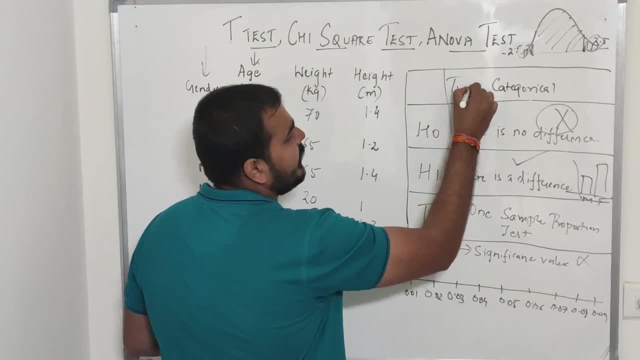 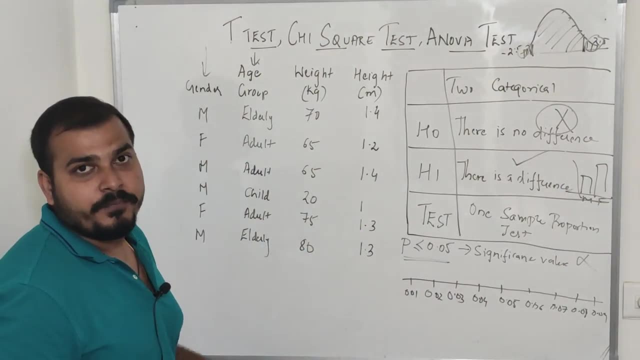 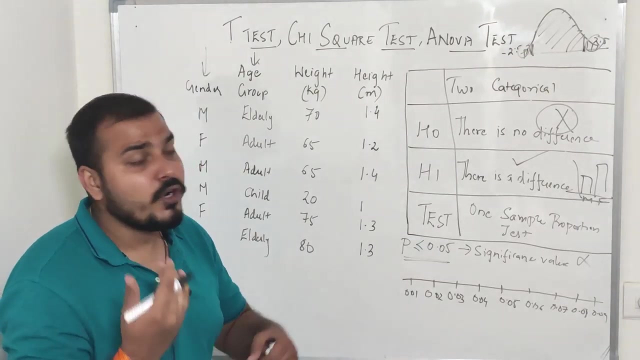 on age group. now this one category become two category, right? okay, now again I can again construct this particular bar plot based on this age group and all, and then again my alternate hypothesis will be that there is a difference and my null hypothesis say that there is no. then there will be no difference, right then? 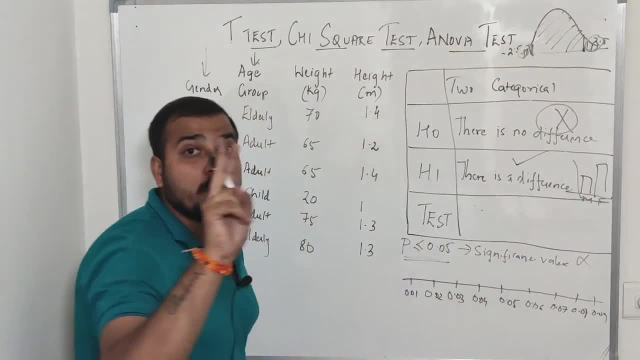 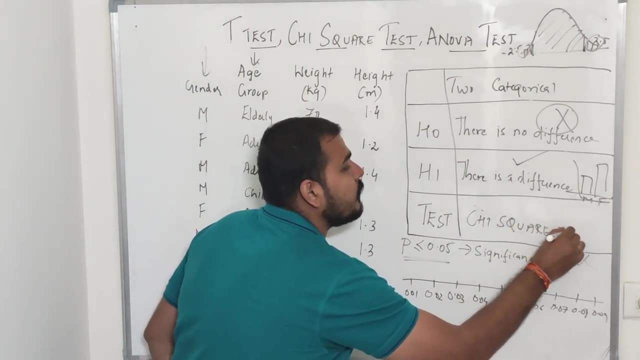 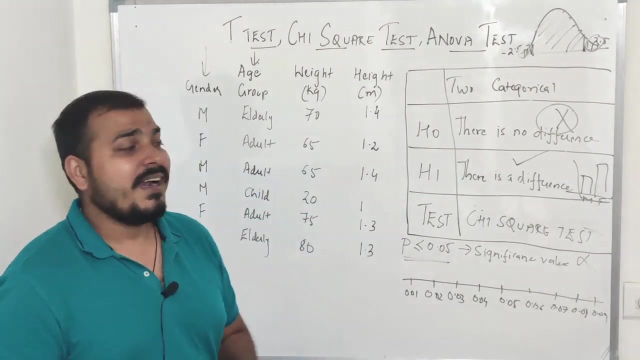 the type of test that we apply if we have two category feature is something called as chi-square test. now, if this chi-square test gives us a value less than 0.05, at that time we are going to consider it that we are going to reject. 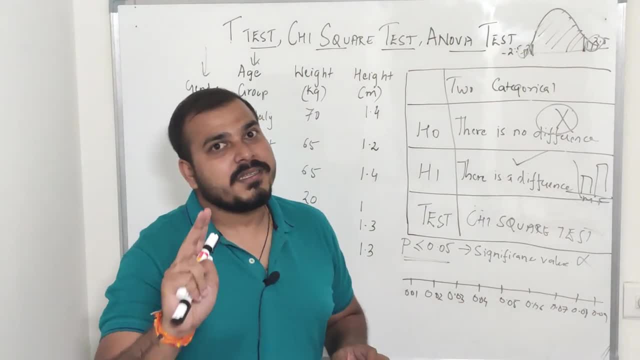 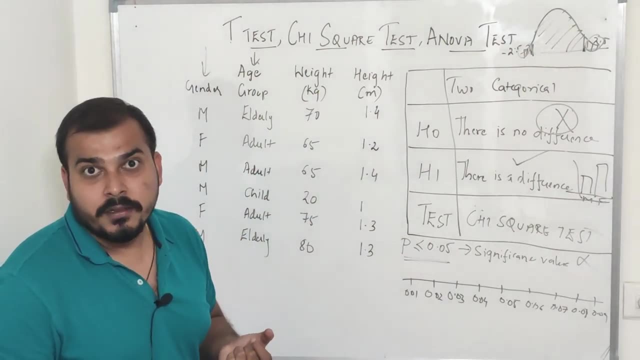 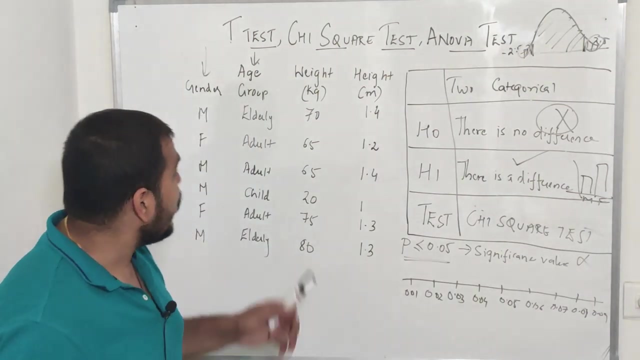 the null hypothesis and accept the alternate hypothesis. always remember this thing, guys: if you are using two category feature and if you're trying to come to a conclusion, like a statement that I've actually told right at that time, you basically have to use a chi-square test. okay, now, now. 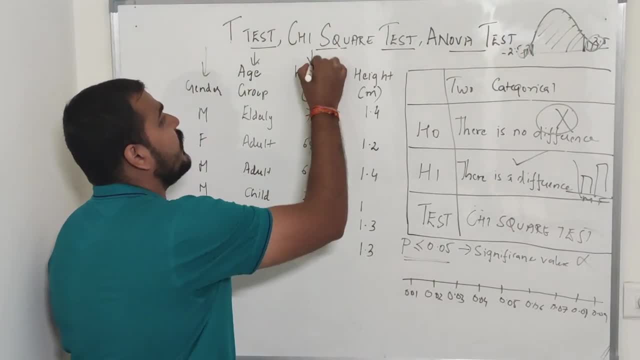 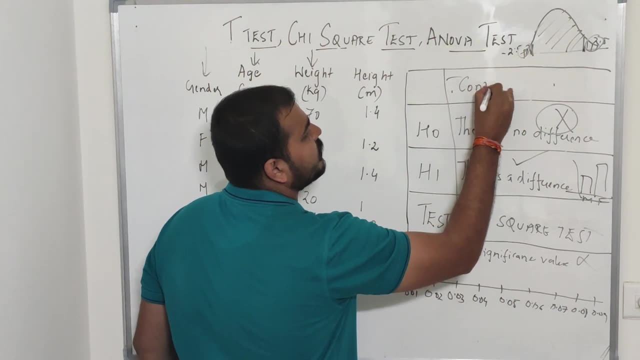 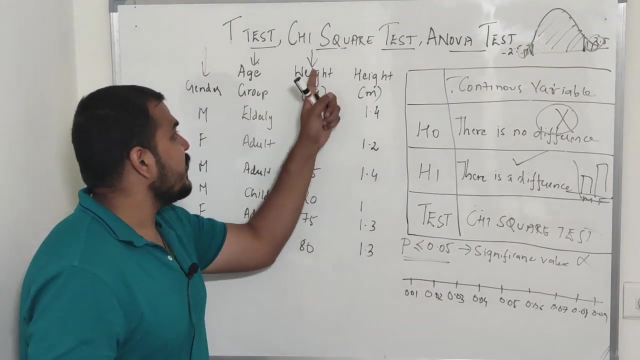 instead of category feature. let me consider one continuous numerical value. okay, now, this two category. I'll just remove it, and let me just say that one continuous variable. now what kind of statement can come up with this with respect to this continuous variable? let me consider that I consider height over here. okay, now, what kind of 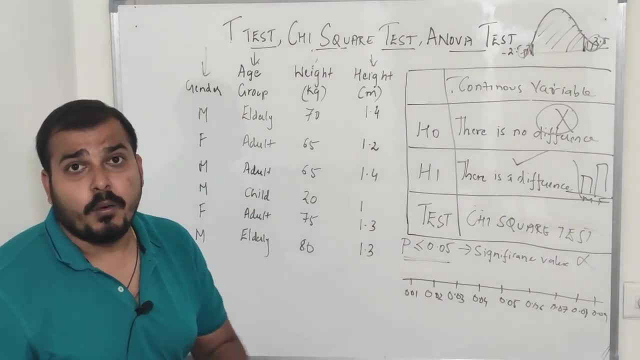 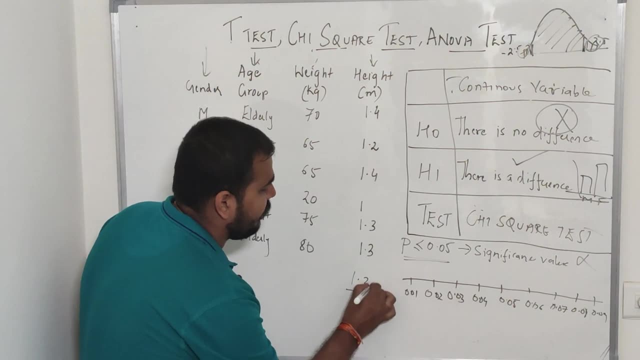 Let me consider that I have considered height over here. Now what kind of statement can I come? Suppose this is my sample height. If I calculate the mean of this height, it may come somewhere around 1.3.. Now I may consider that, based on the previous sample that I have. 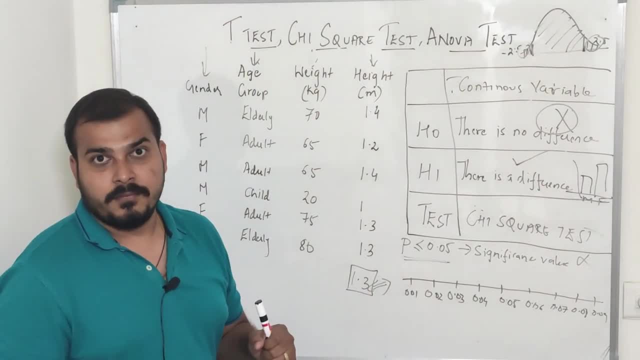 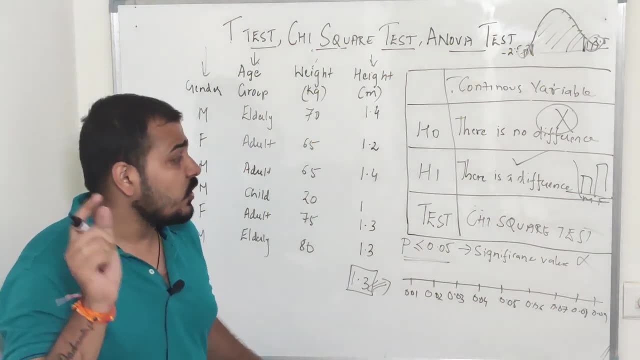 is there a difference with respect to this particular mean height? Again, I can come with this particular statement, Since I just have one continuous variable, continuous feature. So in this case, again, I will write an alternate hypothesis saying that there is a difference. 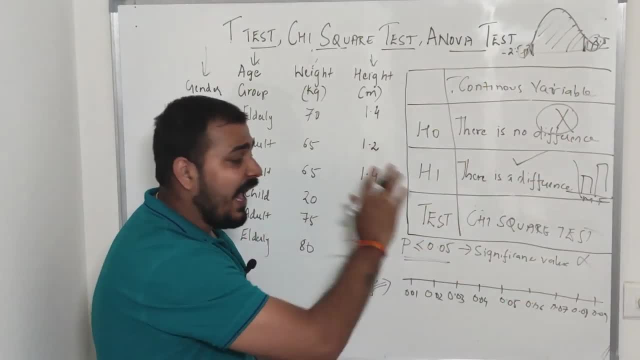 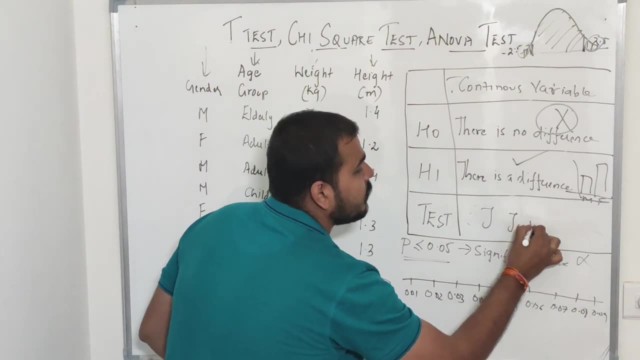 Again, my null hypothesis will be saying that there is no difference And the type of test in case of continuous variable that we basically use is called as t-test. Again, guys, I will be telling you the formula, but just understand the difference. When you have one category feature, you apply one sample proportion test. 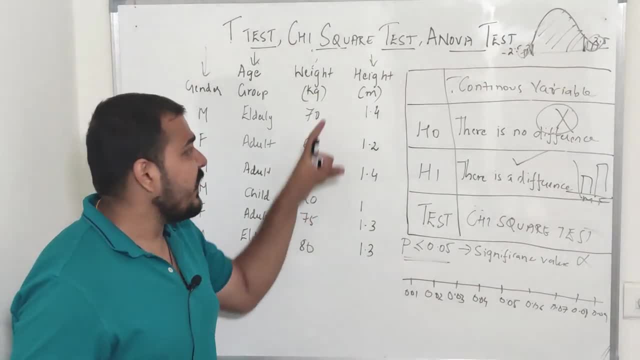 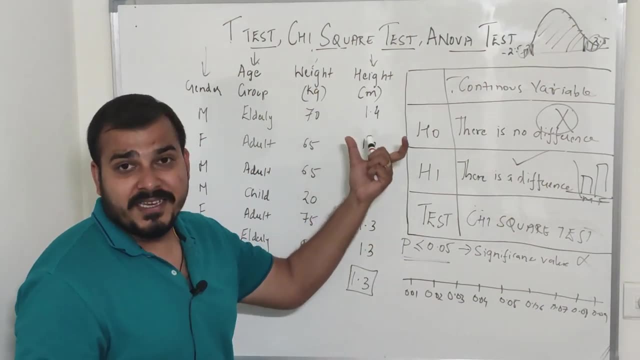 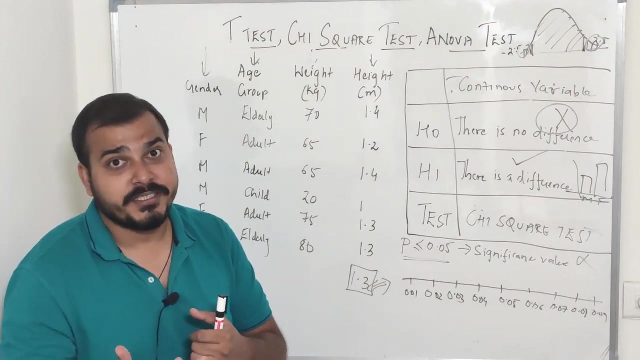 statement. can I come? suppose this is my sample height right? if I calculate the mean of this height, it may come somewhere around 1.3. now I may consider that based on the previous sample that I have, is there a difference with respect to this particular mean height? okay, again, I can come with this particular statement. 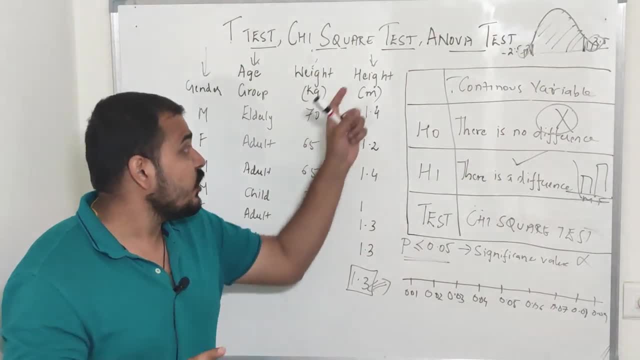 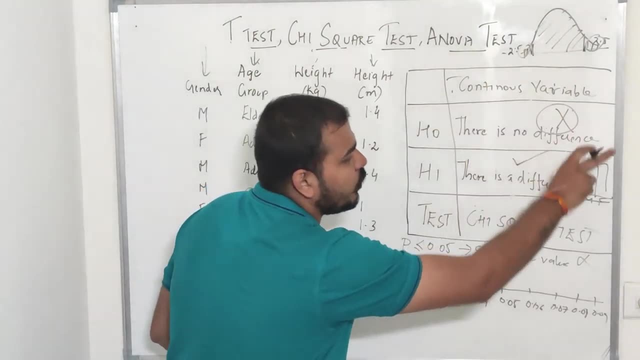 right, since I just have one continuous variable, okay, I can write this in this case. so this case I will write an alternate hypothesis of no difference. again, my null hypothesis will be saying that there's no difference and the type of tests in case of continuous variable that we basically. 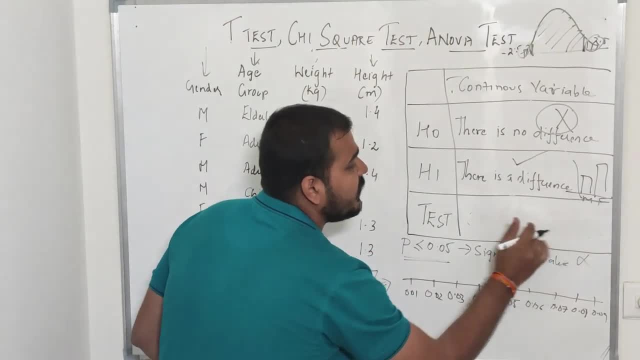 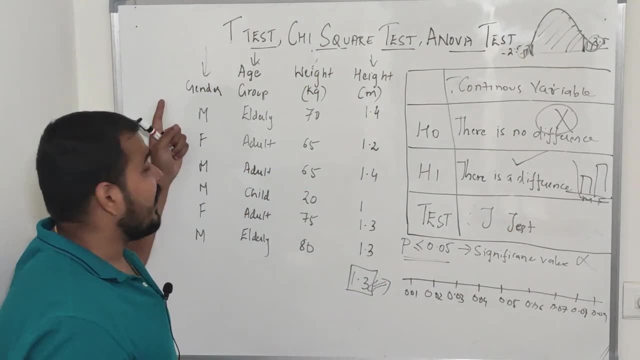 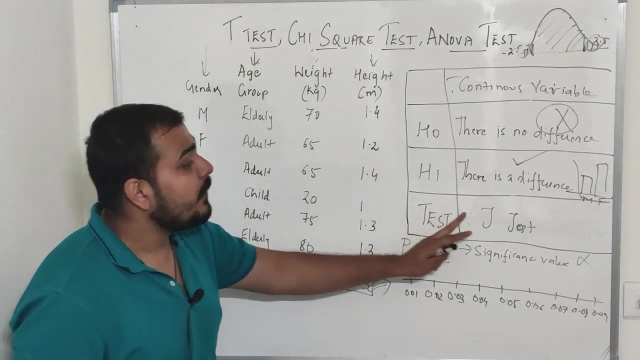 use is called as t test. I'll be telling you the formula, but just understand the difference. when we what kind of feature, you apply one sample proportion test. if you have two category features, you apply chi-square test. if you have one numerical variable, you apply t test- okay. and similarly, if you apply one sample proportion test, okay. 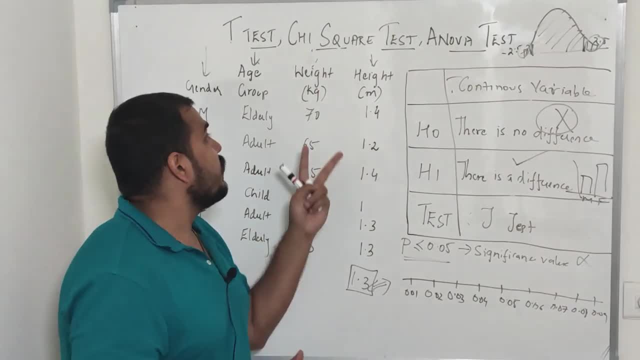 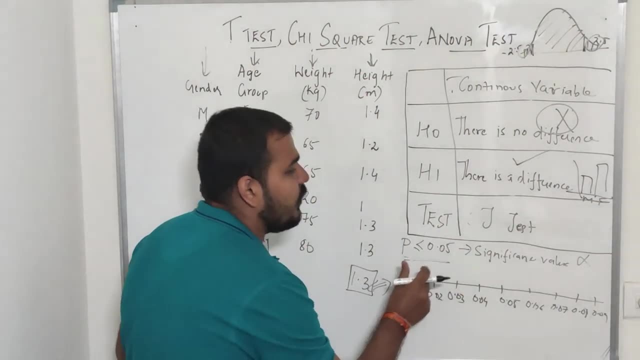 similarly, if you apply two category feature, you apply t test. okay. and similarly, if you apply two category features, you apply t test if you apply two variable. and now let me consider two numerical variable. and again the concept will be same in t test. also, based on this t test, if i get the p value less than 0.05, i am going to 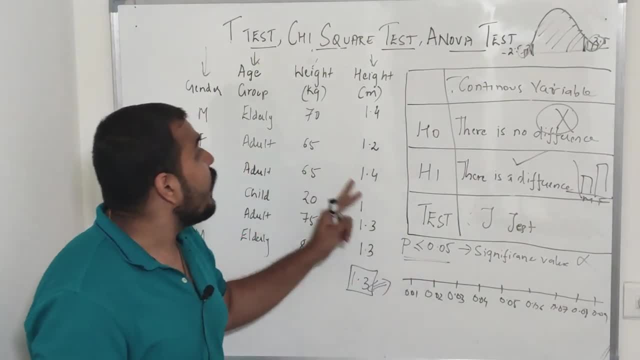 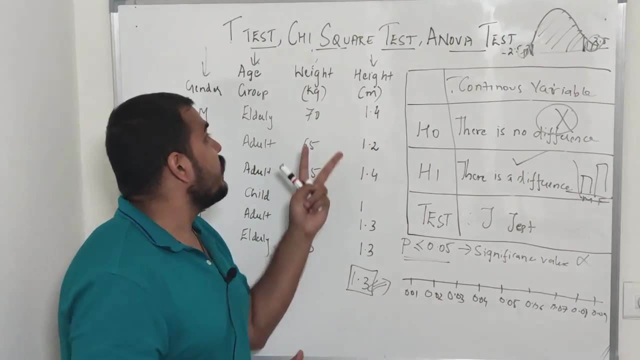 If you have two category feature, you apply chi-square test. If you have one numerical variable, you apply t-test. And similarly, if you apply two categories feature, you apply two variables. and now let me consider two numerical variables. And again, the concept will be same in t-test also. 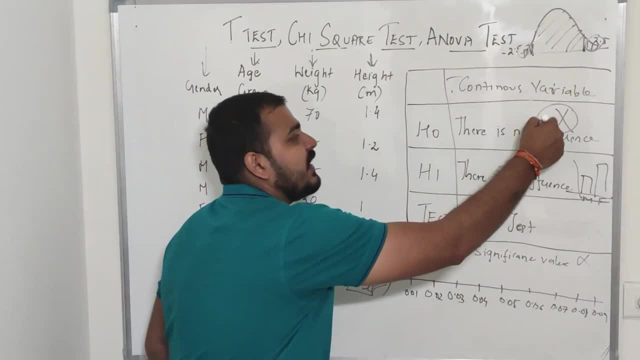 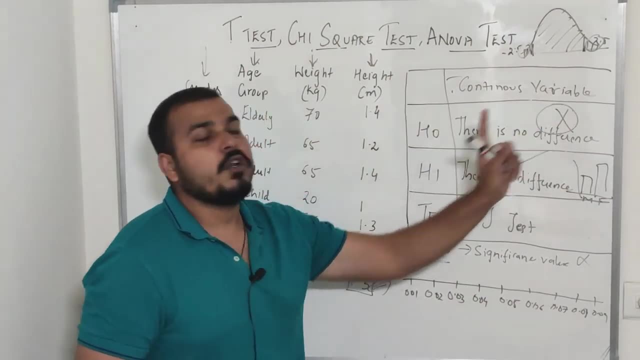 Based on this t-test. if I get the p-value less than 0.05, I am going to reject the null hypothesis and I am going to accept the alternate hypothesis. If the p-value is greater than 0.05, I am going to stay true with this. 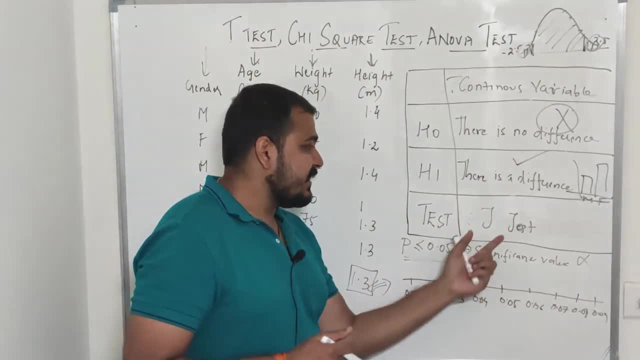 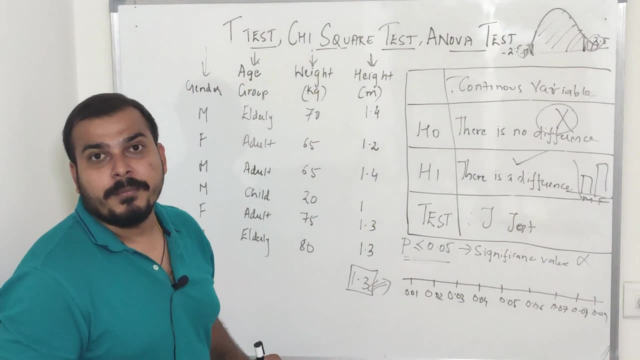 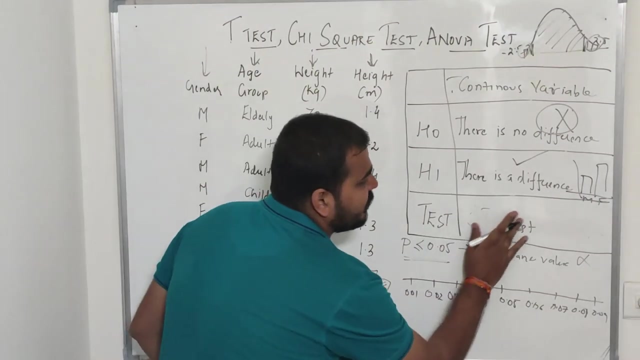 That is my null hypothesis, saying that there is no difference. And again, this test formula I will be defining in the next class itself. Now suppose, if I consider two numerical variables, What kind of test we can apply For this? we basically apply a test which is very, very common and everybody knows it. 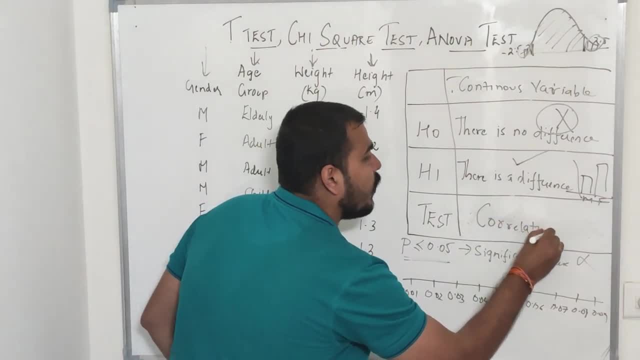 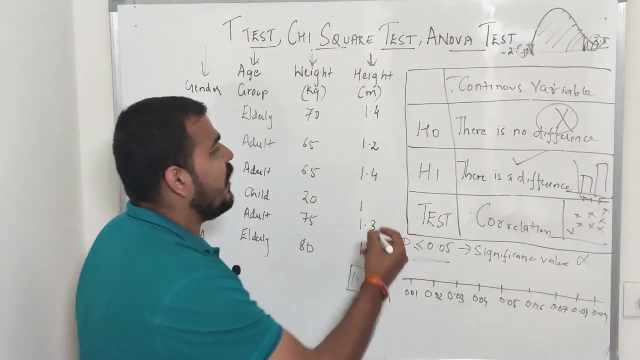 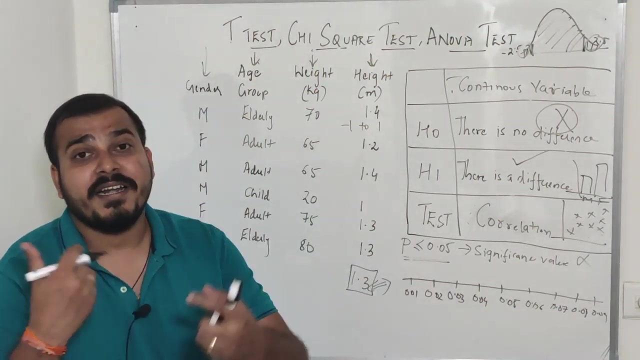 Which is called as correlation. Now, what is this correlation? We create this kind of graph. Let me try to see this correlation. And according to Pearson correlation, the value always ranges between 1 to minus 1 to plus 1.. If there is no correlation, suppose, how do I determine the two features are not having correlation? 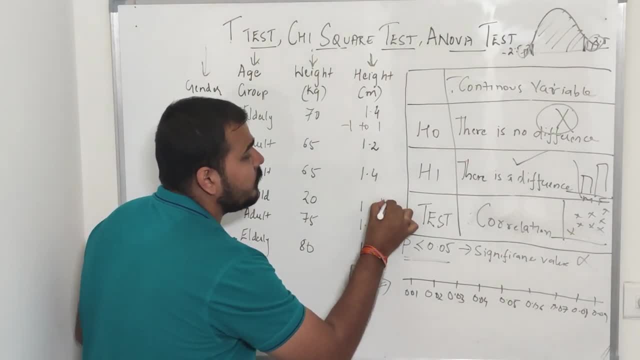 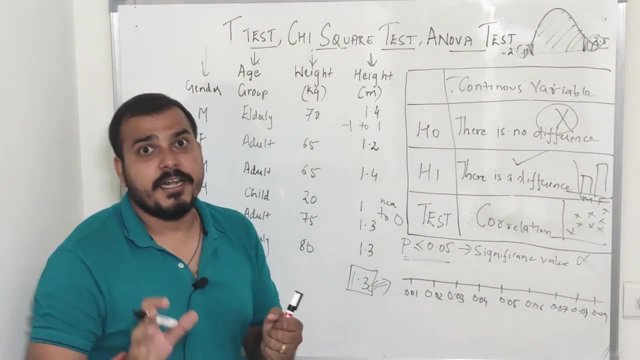 That basically means that our correlation value will be somewhere near to 0.. If it is near to 0, it basically indicates no correlation. I hope you have seen my video on Pearson correlation, So just understand in this particular way that if my correlation is somewhere near to 0,. 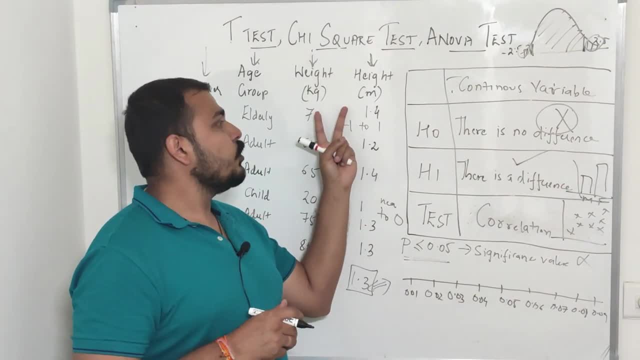 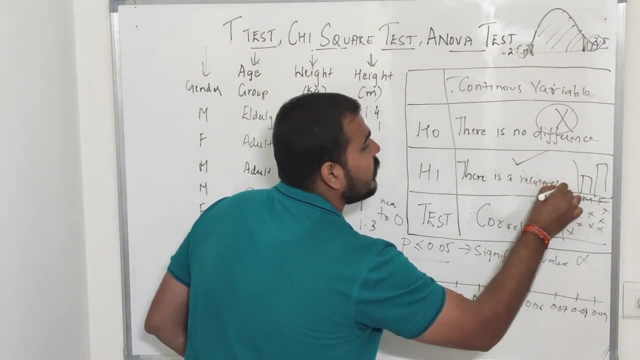 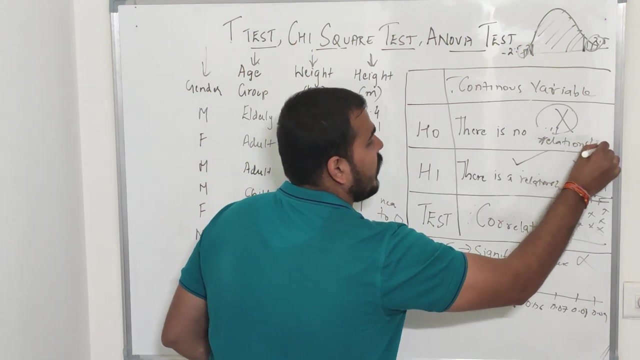 that basically indicates that there is no relationship between this particular numerical variable. Now I can just say that there is a relationship over here. as my alternate hypothesis In the null hypothesis, I can say that there is no relationship Again. now, based on this, we can again apply a t-test. 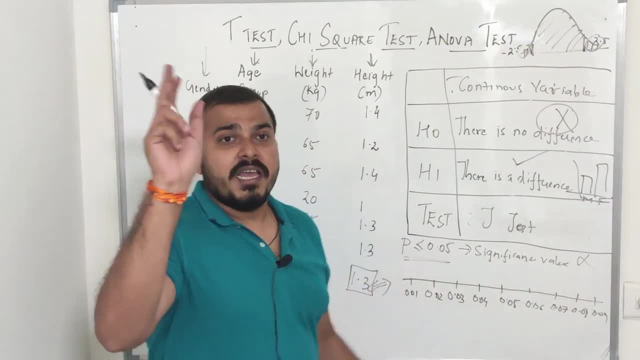 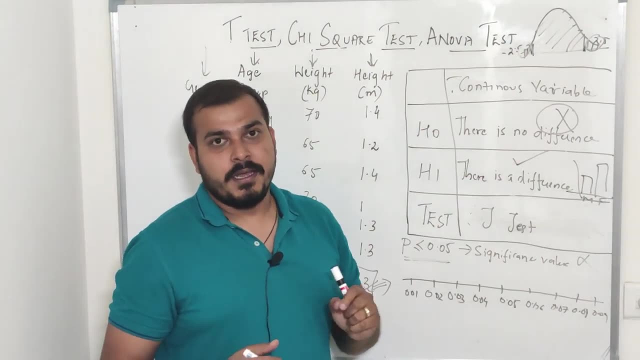 reject the null hypothesis and i am going to accept the alternate hypothesis if the p value is greater than 0.05. i am going to stay true with this. that is my null hypothesis, saying that there is no difference. and again, this test formula i will be defining you in the next class itself. 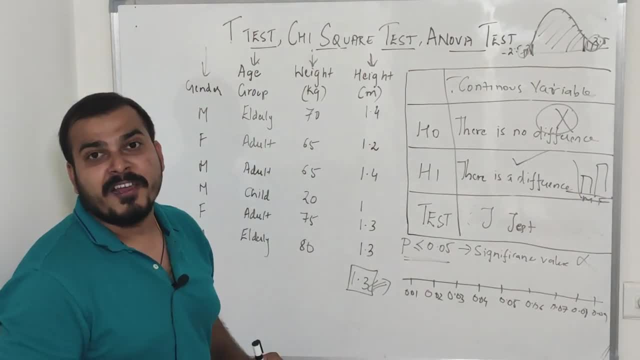 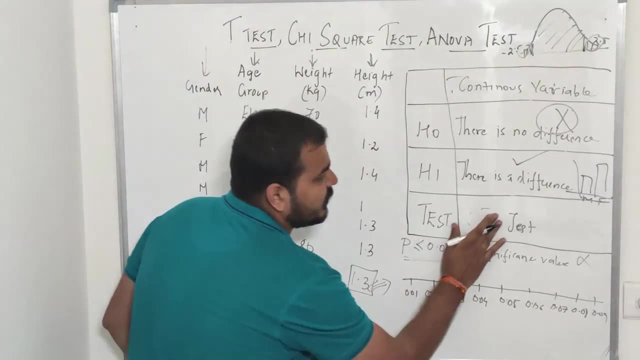 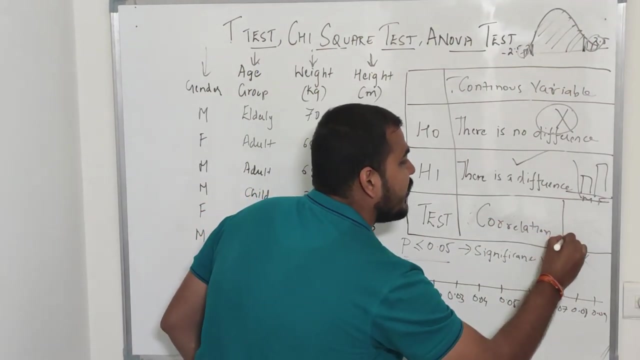 okay, now suppose, if i consider two numerical variable- now two numerical variable over here- what kind of test we can apply for this? we basically apply a test which is very, very common and everybody knows it, which is called as correlation. now, what is this correlation? we create this kind of graph. let me try to see this correlation right and according to pearson, 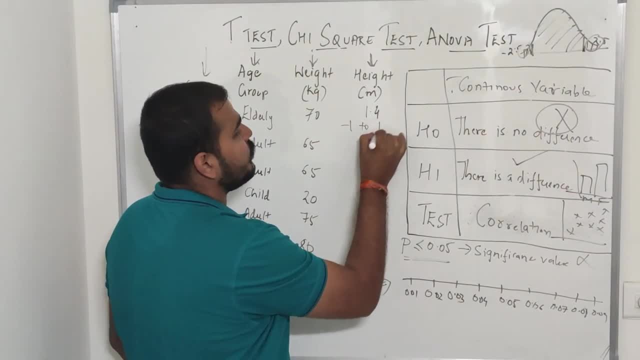 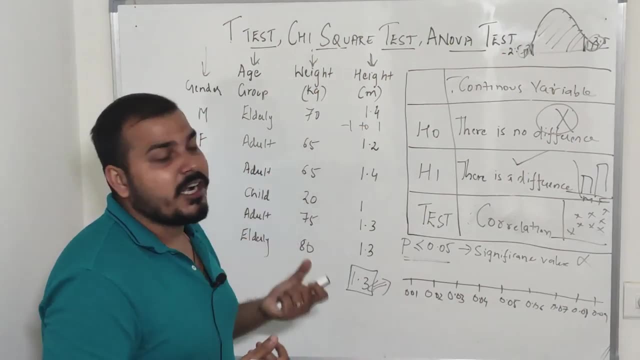 correlation. the value always ranges between 1 to minus 1 to plus 1, right, if there is no correlation? suppose if there is no correlation, then what is the correlation between 1 to minus 1 to plus 1? suppose. how do i determine the? the two features are not having correlation. that basically means: 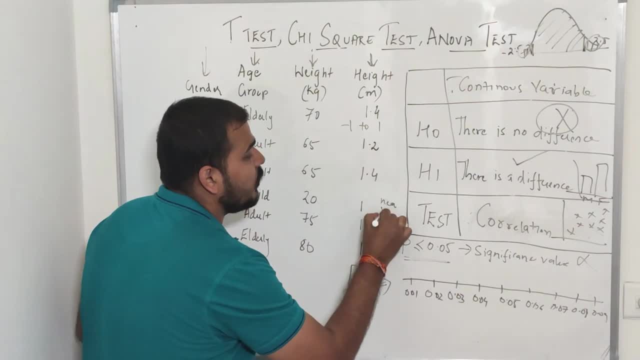 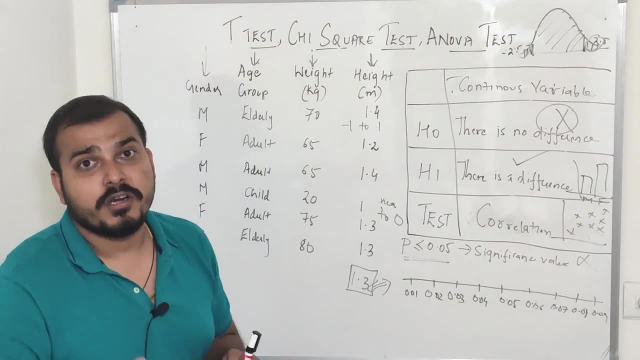 that our correlation value will be somewhere near to 0, right? if it is near to 0, it basically indicates no correlation, right? i hope you have seen my video on pearson correlation, so just understand in this particular way that if my correlation is somewhere near to 0, 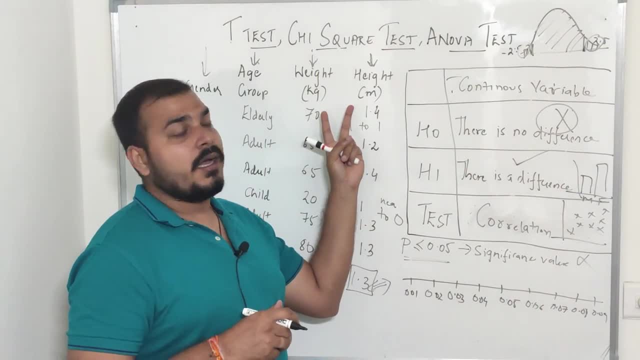 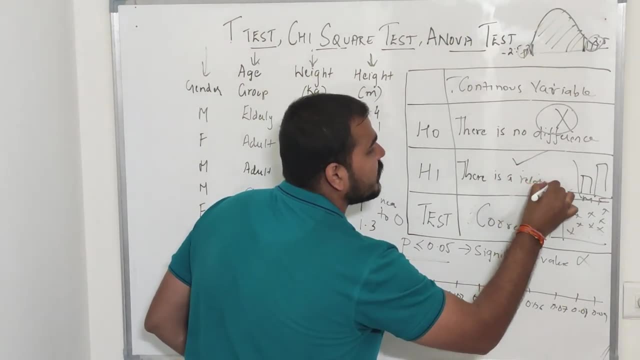 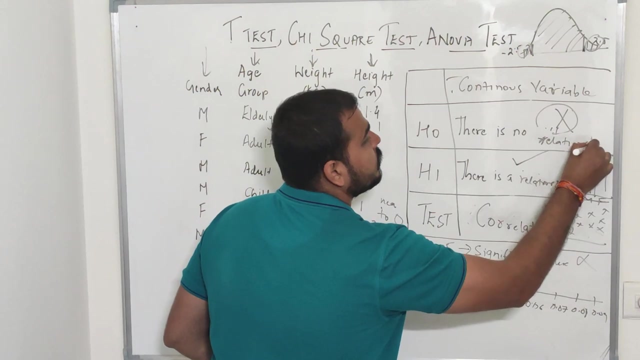 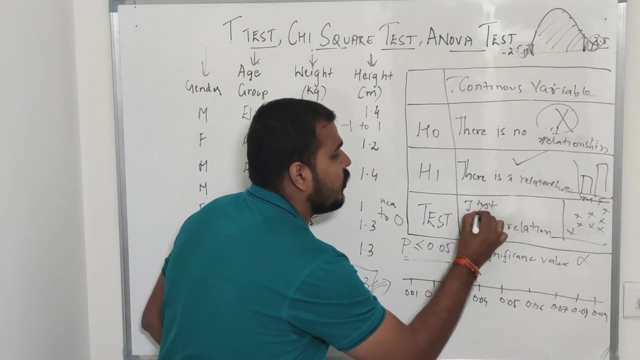 that basically indicates that there is no relationship between this particular numerical variable. now i can just say that there is a relationship over here. as my alternate hypothesis in the null hypothesis i can say that there is no relationship. again, now, based on this, we can again apply a t test and we can come to a conclusion saying that 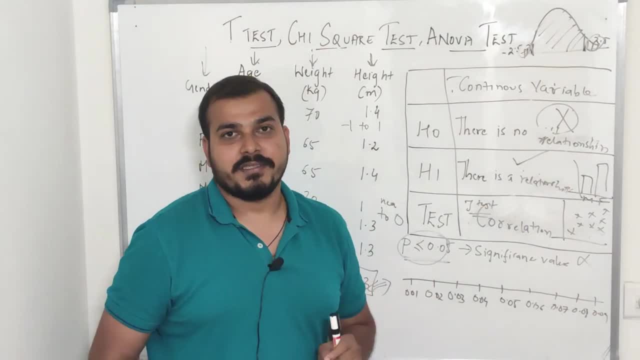 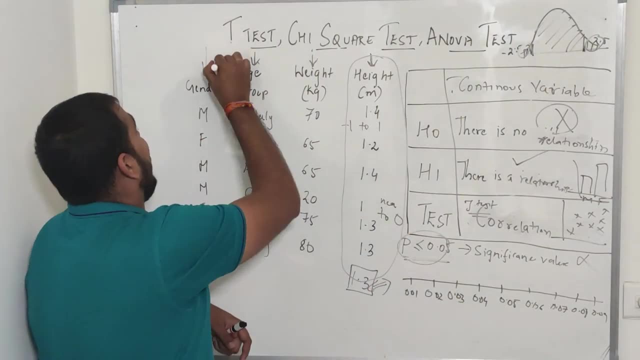 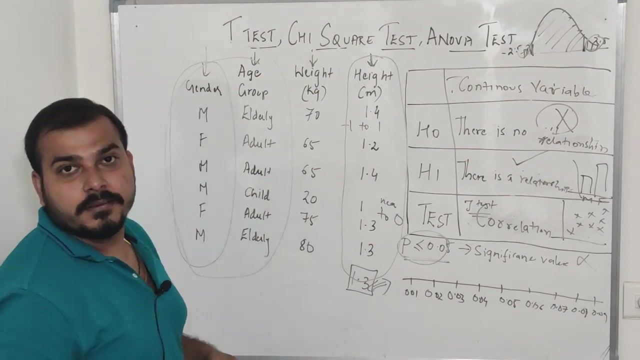 my p value is less than this, i am going to reject it, otherwise i am going to accept this. okay, now, guys, one more thing. suppose i consider one numerical variable and one category variable, or two category variable, or category variable which has more categories, which has more categories. over here you can see that it is having more than two categories. we have elderly, we have 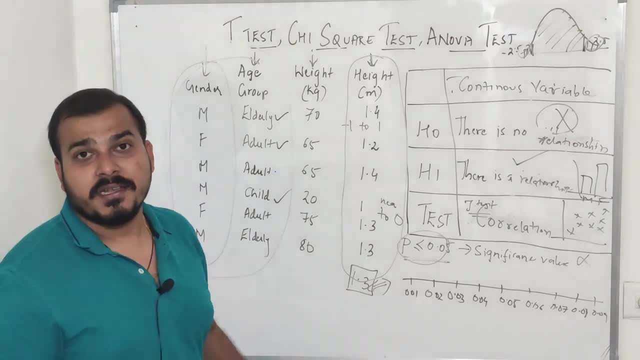 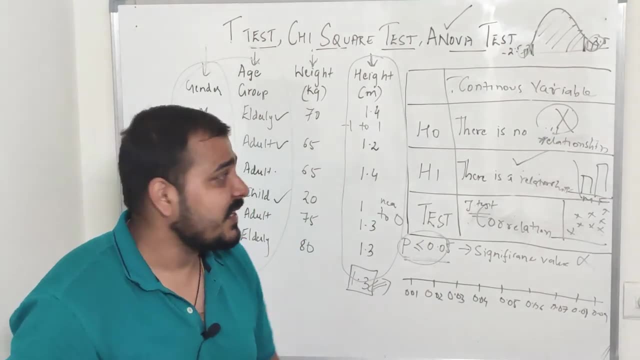 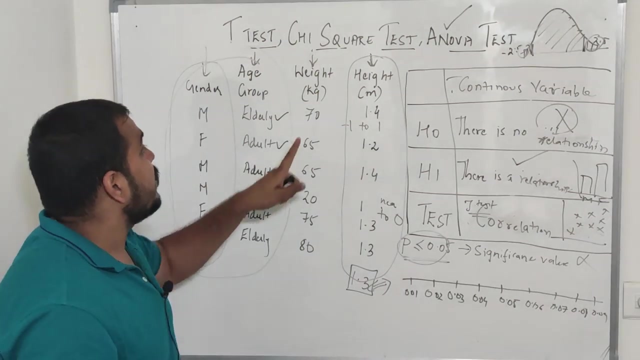 adult, we have child, right? if it is having more than two categories, then what kind of test we basically apply is called as anova test. okay, again, guys just understand these things. because based on the num, based on the category feature, based on the numerical feature. now, when do we apply anova test? is that suppose, if i have a scenario wherein 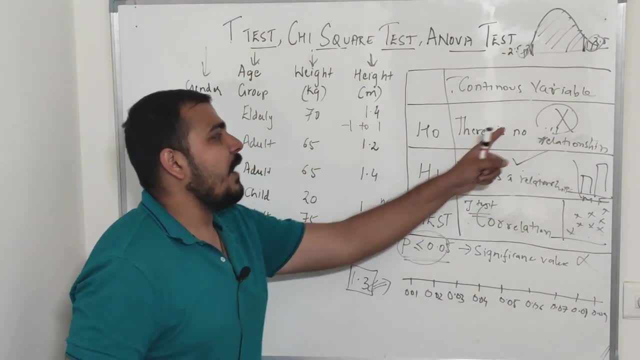 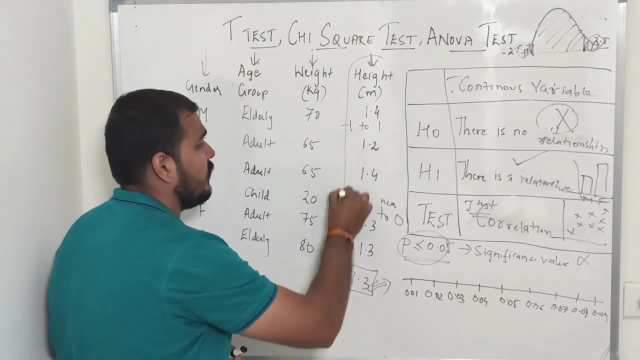 And we can come to a conclusion saying that if my p-value is less than this, I am going to reject it. Otherwise I am going to accept this. Now, guys, one more thing. Suppose I consider one numerical variable and one category variable. 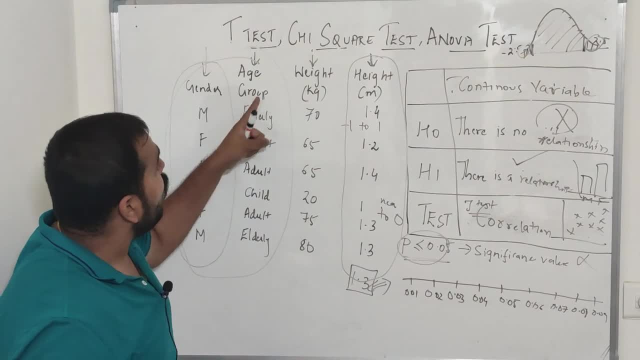 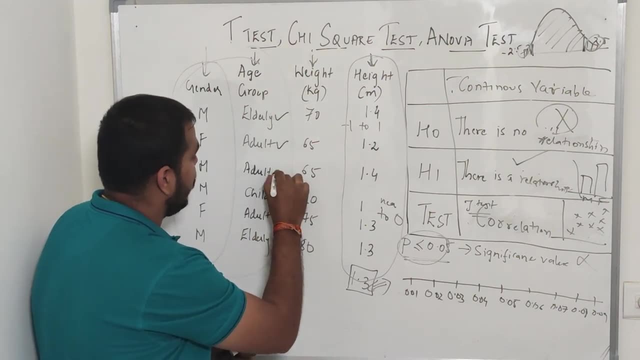 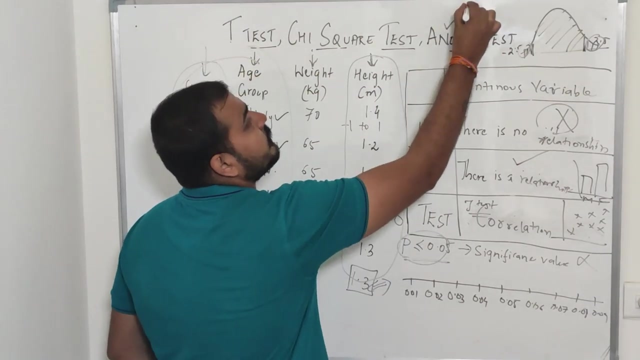 Or two category variables, And I consider a variable which has more categories, Which has more categories over here You can see that it is having more than two categories: We have elderly, we have adult, we have child. If it is having more than two categories, then what kind of test we basically apply is called as ANOVA test. 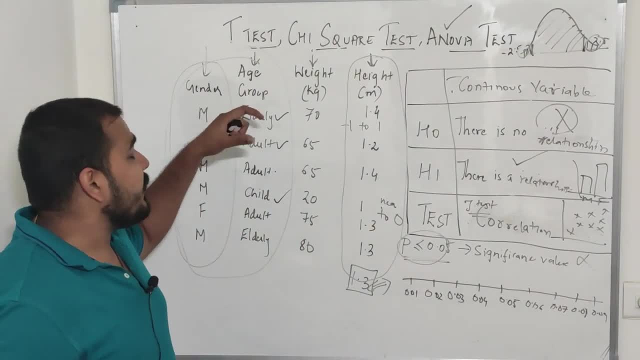 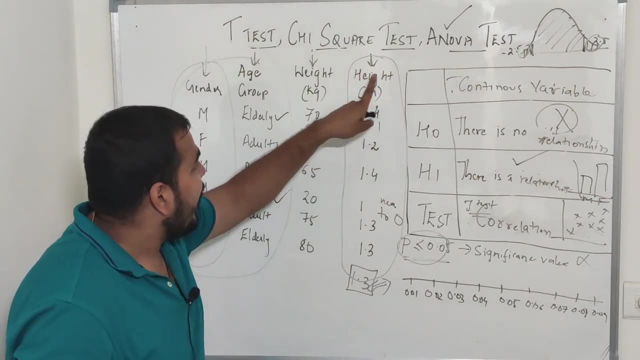 Again, guys just understand these things. because based on the categorical feature, based on the numerical feature. now when do we apply ANOVA test? is that suppose if I have a scenario wherein I have a numerical variable and I have a category variable? 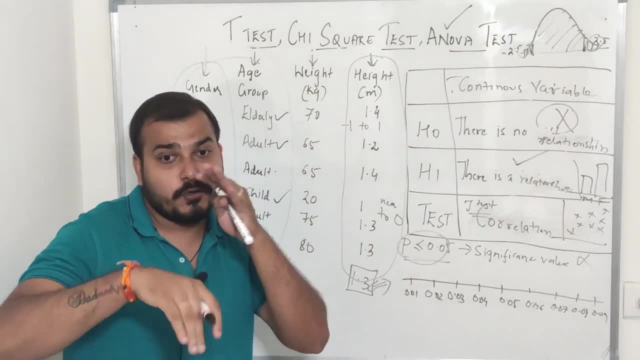 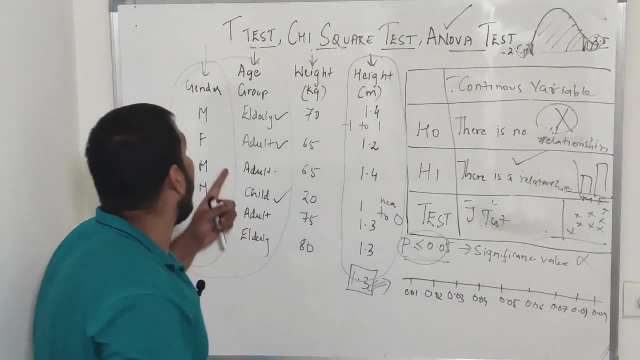 And suppose in this particular category variable I have two categories only, At that time I apply only t-test, I apply only t-test. Suppose if I have a category feature which has more than two categories, then I go with ANOVA test. 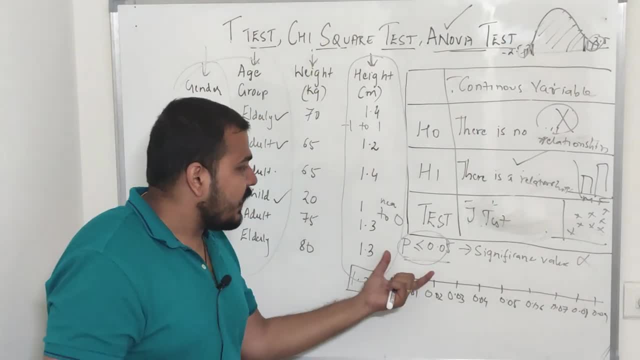 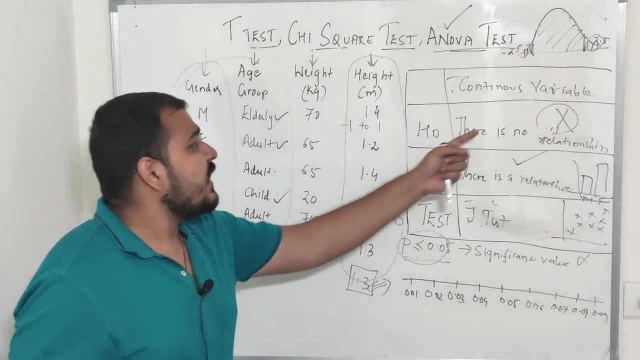 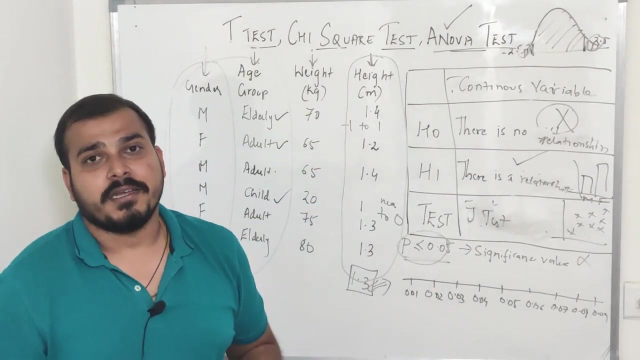 And again, the methodology will be same guys- That whenever, through this particular test, we get a value p is less than or equal to 0.05, we are going to basically reject our null hypothesis and accept our internet hypothesis. If it is greater than 0.05, we are going to accept the null hypothesis and reject the alternate hypothesis. 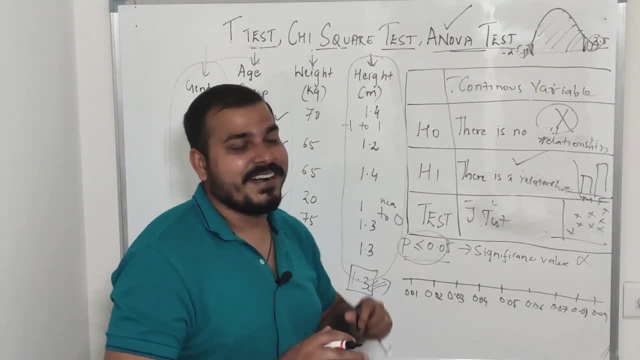 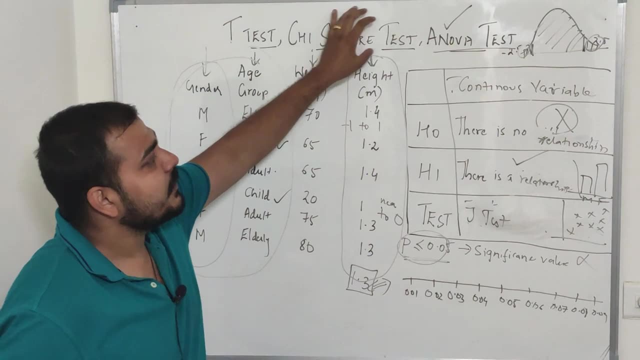 Right, Sorry, We should accept the null hypothesis and reject the alternate hypothesis. So, yes, this was all about this particular video. I hope you have understood. when do we use t-test? when do we use calcuer test? when do we use ANOVA test? 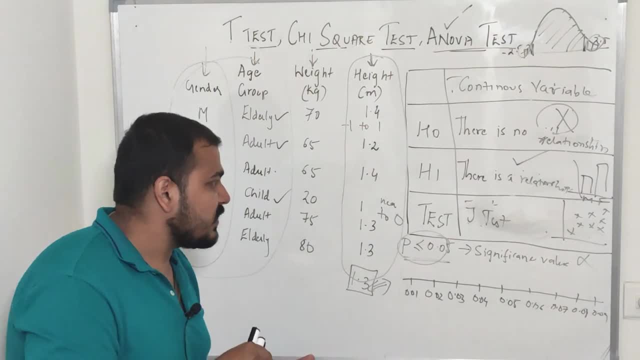 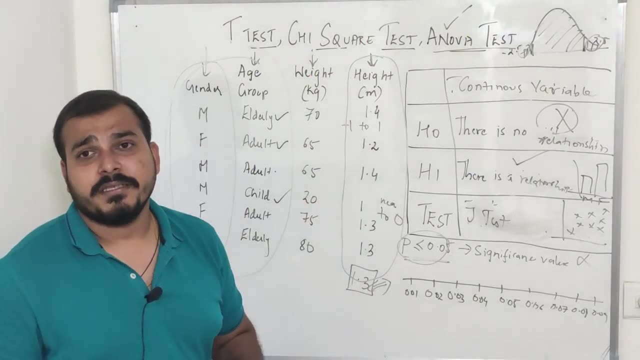 And this is the fundamental mechanism behind hypothesis testing and the type of test you do. In my upcoming videos, I am going to show you an example with the help of python programming language. How do you perform this particular test, And that time you will be able to understand, with respect to code also. 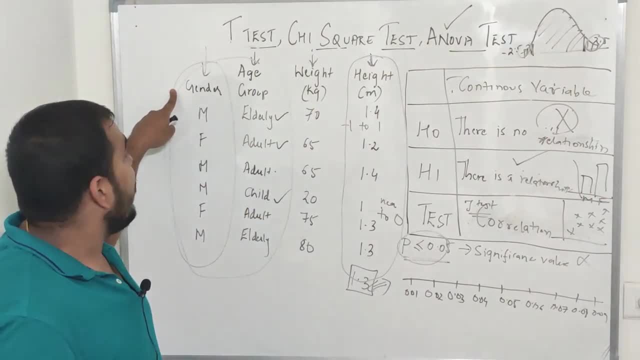 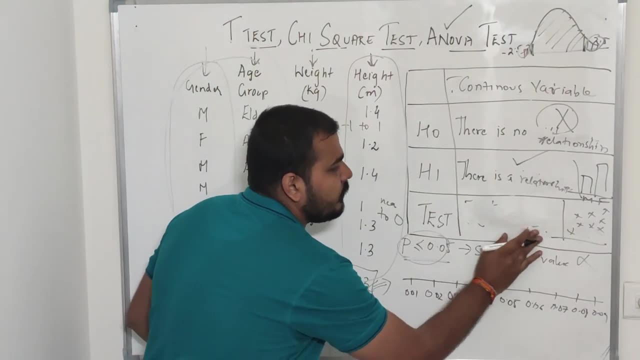 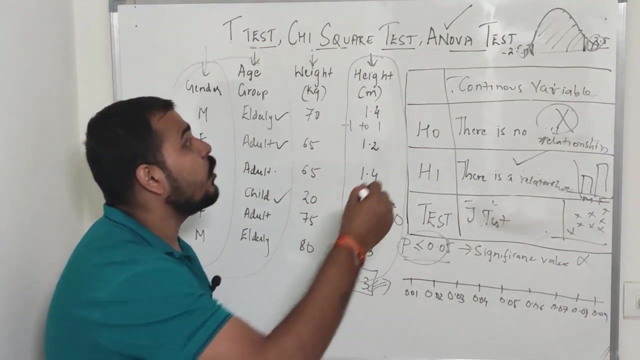 i have a numerical variable and i have a category variables and suppose in this particular category variable i have less. i have, i have two categories. only at that time i apply only t test. okay, i apply only t test. suppose if i have a category feature which has more than two categories, then i go with. 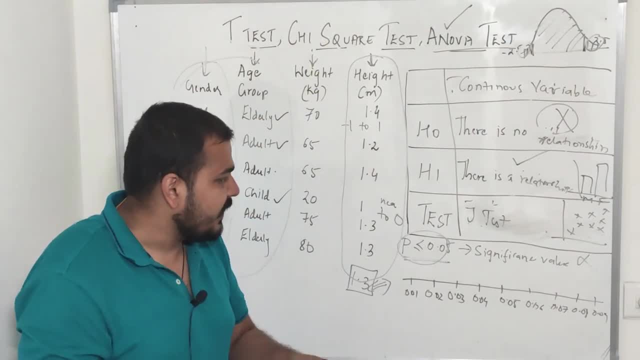 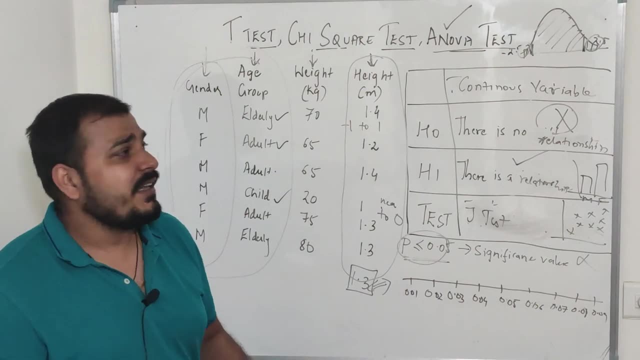 anova- and again, the methodology will be same, guys- that whenever, through this particular test, we get a value p is less than or equal to 0.05, we are going to basically reject the normal hypothesis and accept our alternate hypothesis. if it is greater than 0.05, we are going to accept. 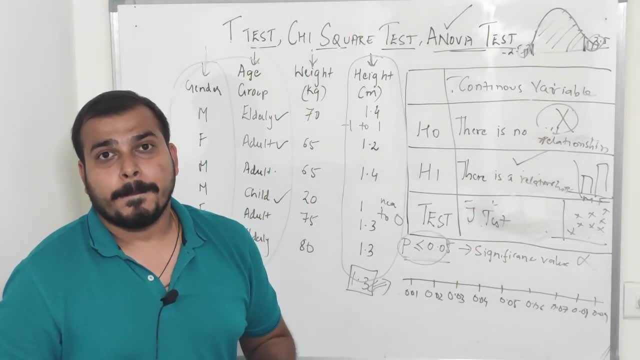 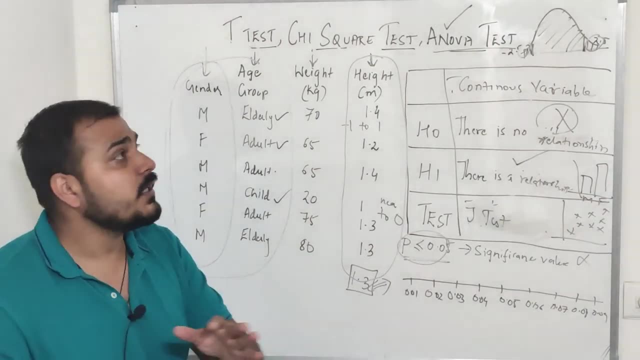 the null hypothesis and reject the null hypothesis. right, sorry, we should accept the null hypothesis and reject the alternate hypothesis. so, yes, this was all about this particular video. I hope you have understood. when do we use t-test? when do we use calcule test? when? 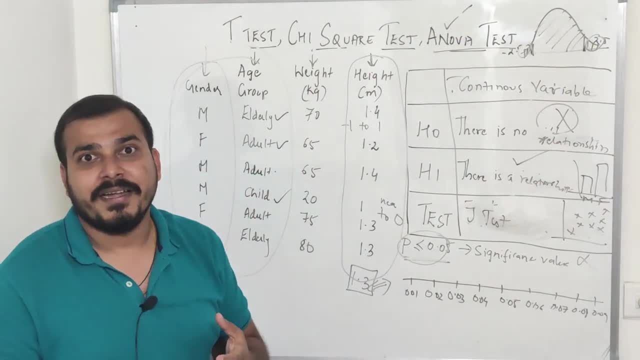 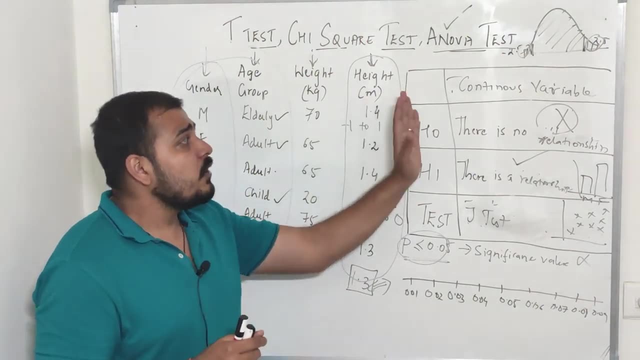 do we use ANOVA test, and this is the fundamental mechanism behind hypothesis testing and the type of test you do. in my upcoming videos, I am going to show you an example with the help of python programming language. how do you perform this particular test and that.